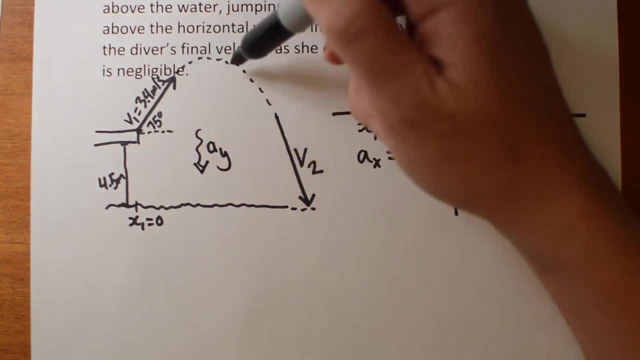 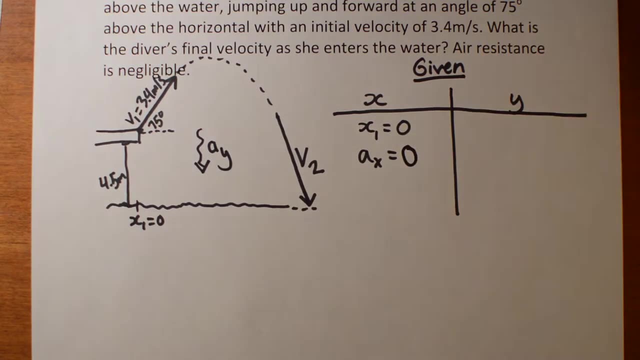 is just feeling the force of gravity, So they'll go up and accelerate downwards. There's nothing pulling them forwards at all, So that acceleration in the x direction is just zero. I should toss, by the way on my picture, a little coordinate system: Y is positive up, X is positive. 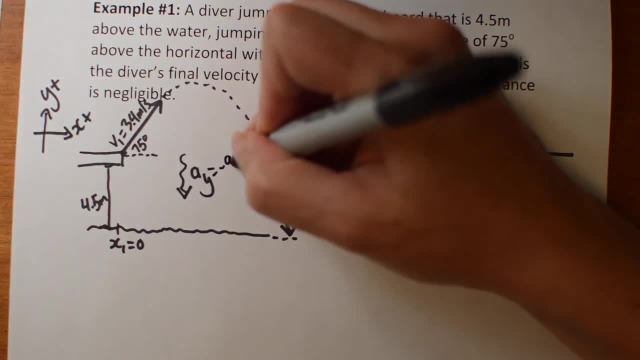 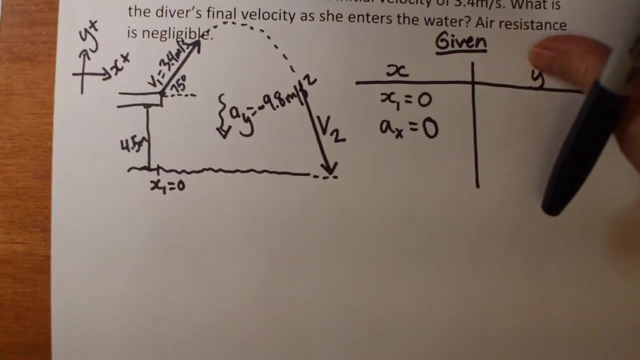 forwards And that's going to make this ay a negative 9.8 meters per second squared. So it's important to have my coordinate system to make sure I'm getting my signs right here, All right. one more thing: I know in the x direction and that is my initial velocity. So v1 in the x. 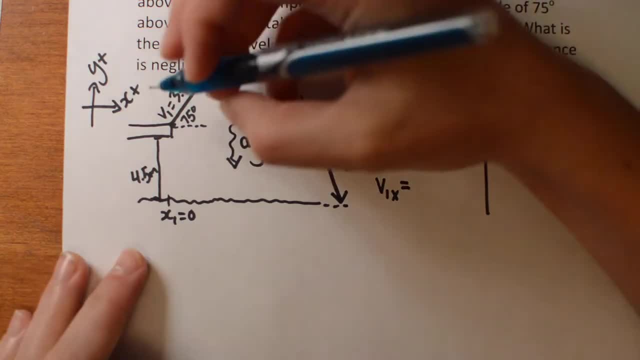 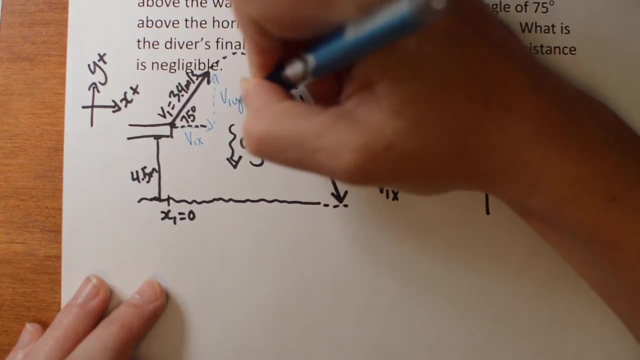 direction, Which I'm going to need a little Sakatoa for, So I can split this up into a right angle triangle right. Here's v1 x. Here's v1 y, If you remember from our video reviewing Sakatoa. 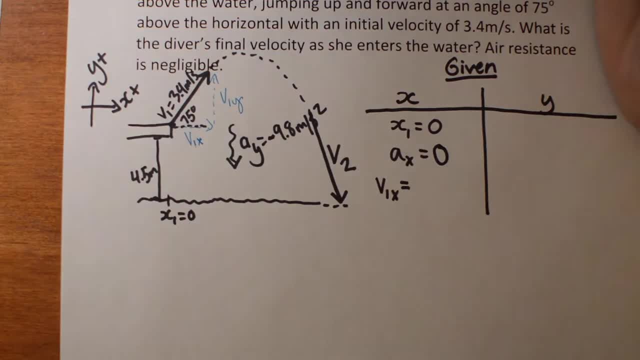 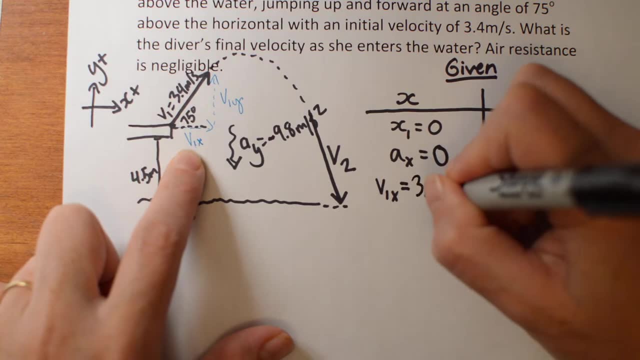 there's a quick trick we can use here where we can say that cos is close, So v1 x is close to our 75 degree angle, So it's going to be the 3.4, the hypotenuse times, cos of 75. And then toss it in my 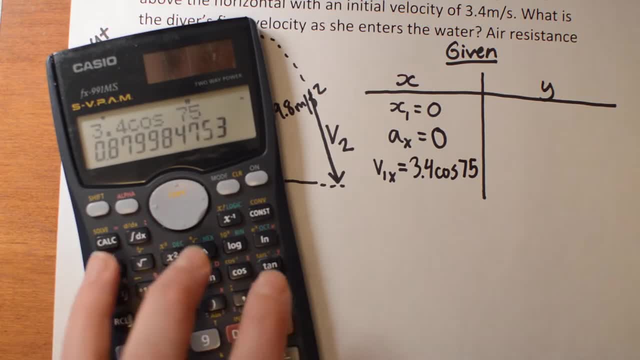 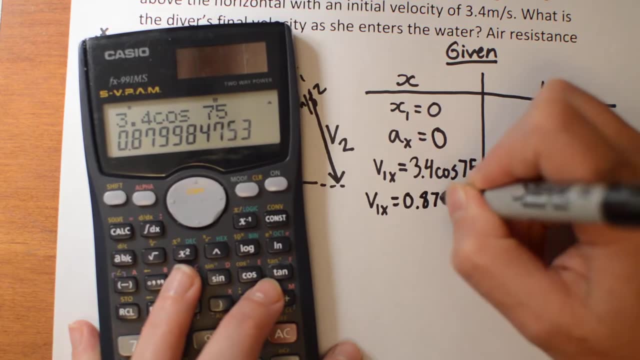 calculator 3.4 cos of 75.. At this stage it's a good idea to just write down a gazillion decimal places in your answer. It seems a little unnecessary, but it'll be useful. So I'm just going to pick that up and I'm going to use this as my form for the next step. So if you're at the видите, we've got to say: 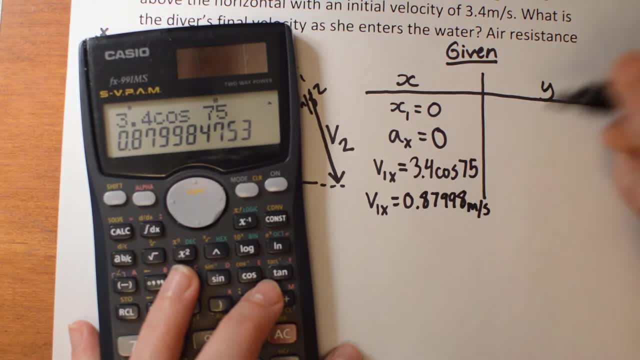 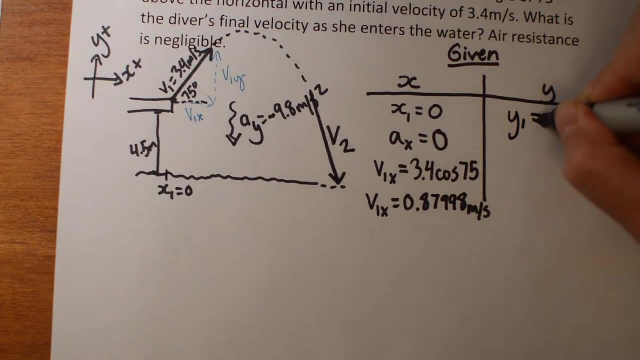 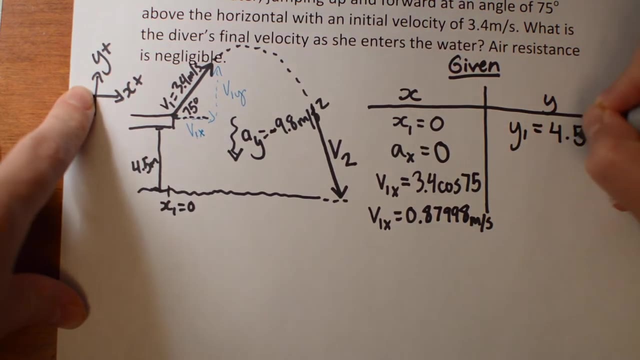 just prevent any accidental rounding errors. so write down five decimal places. it's way more than enough. all right, why information stuff? um, so for y, if we think about our y1, that's my initial height that i start off at, and this diver starts off at 4.5 meters above the ground right or above the. 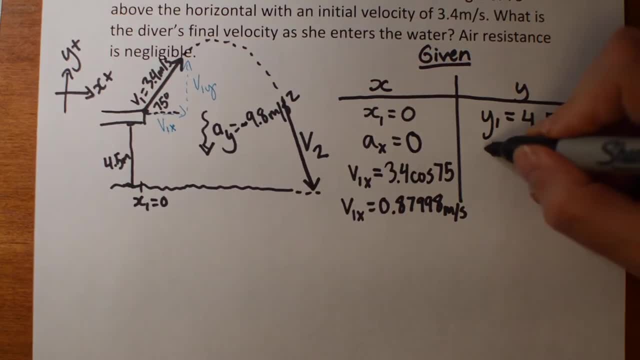 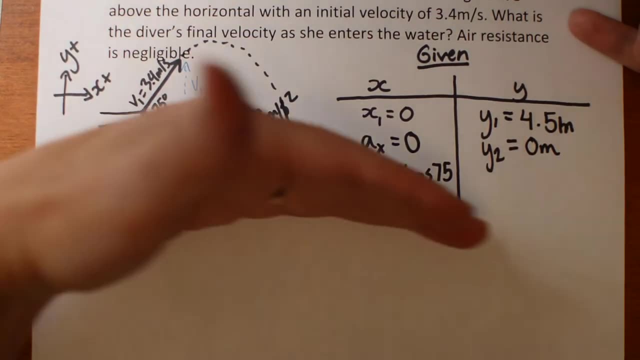 water. so 4.5 meters is my initial height and i also know the final height when the diver is entering the water has a height of zero at the water. so we've kind of defined y equals zero to be the water point. i know the acceleration in the y direction, that's the acceleration due to gravity. 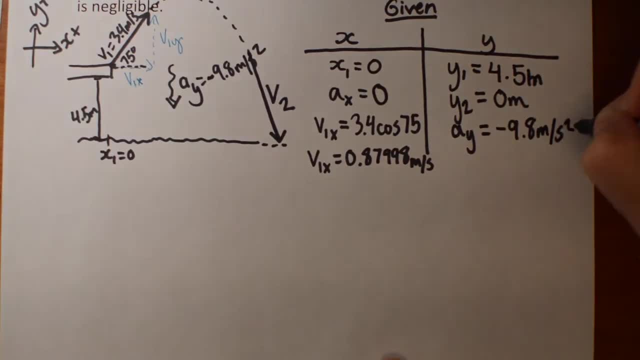 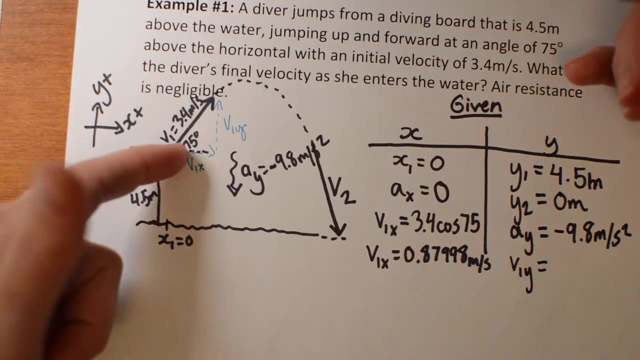 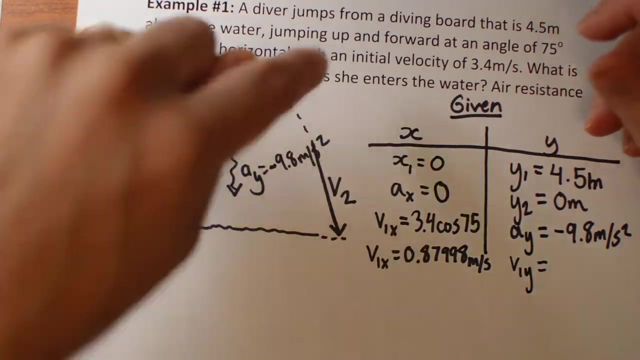 so that'll be negative 9.8 meters per second squared and i know v1 in the y direction. so if we remember from that video a little while ago, sine is far away, like signs on the highway are far away. so the v1y is opposite my 75 degree angle. it's very far away. it's going to be 3.4 sine of. 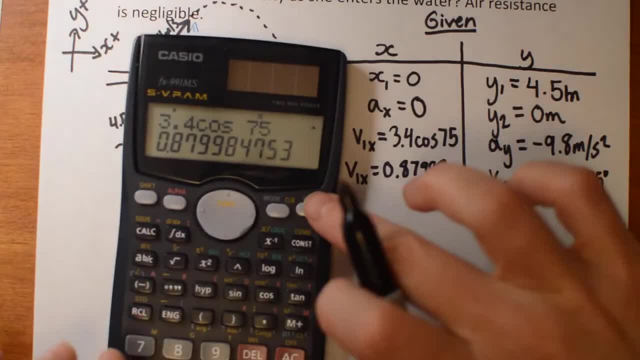 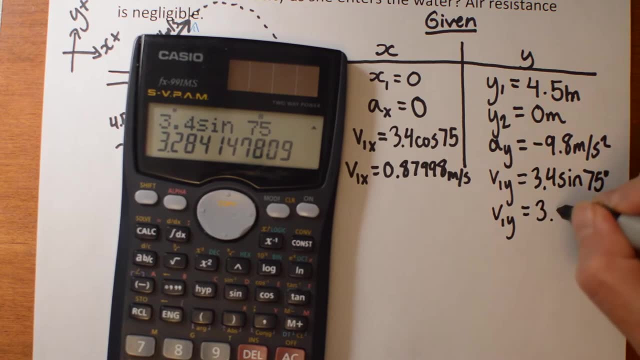 that 75 degree angle. it's going to toss that in your calculator. 3.4 sine 75 and we get v1y is 3.28415. that's plenty meters per second. okay, great, that's basically everything i'm given. what am i looking for? so? 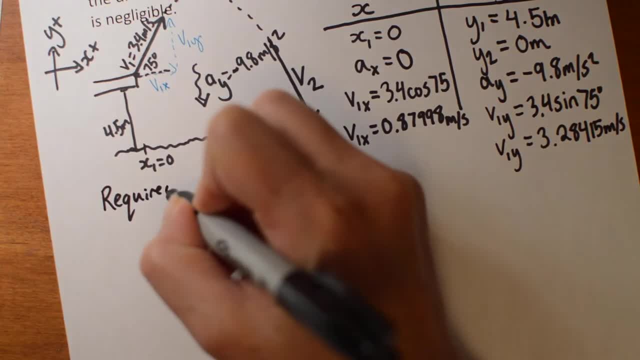 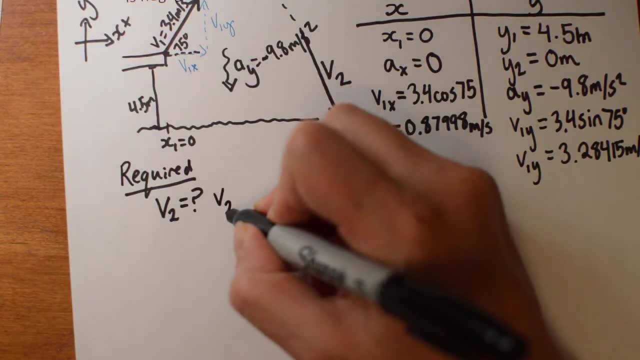 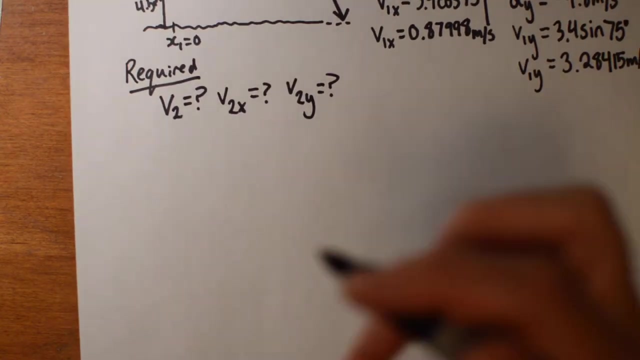 my required put over. here i'm trying to find v2, which means that i need to find v2, the velocity in x direction, and the final velocity in the y direction. let's start with the x direction. so v2x is actually really straightforward. here we're not accelerating. 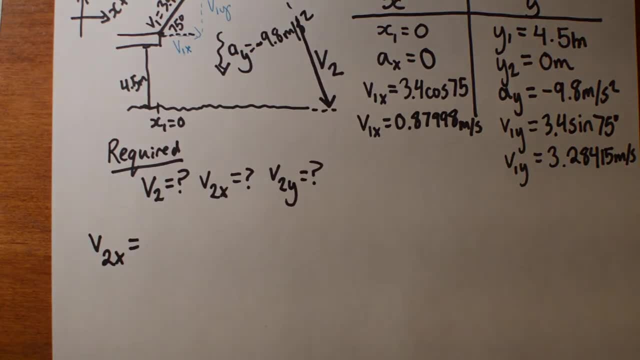 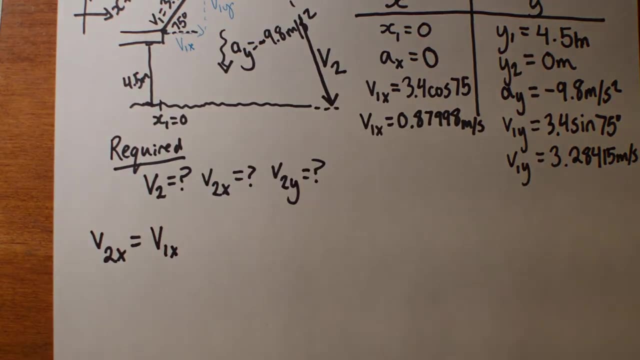 in the in the x direction at all right, we're not speeding up or slowing down. that means that v2x is just equal to v1x. the diver is going the same speed horizontally through that entire jump. if you want to sort of prove that to yourself, you can use the first kinematics equation, which is: 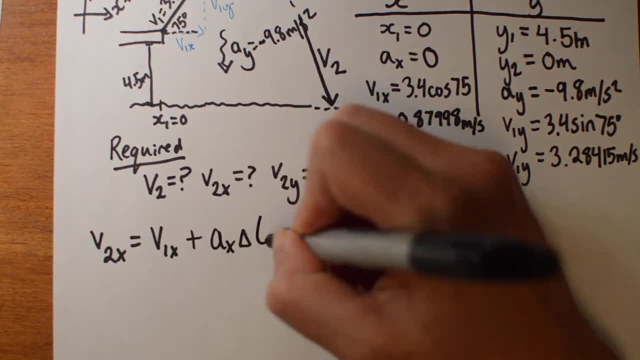 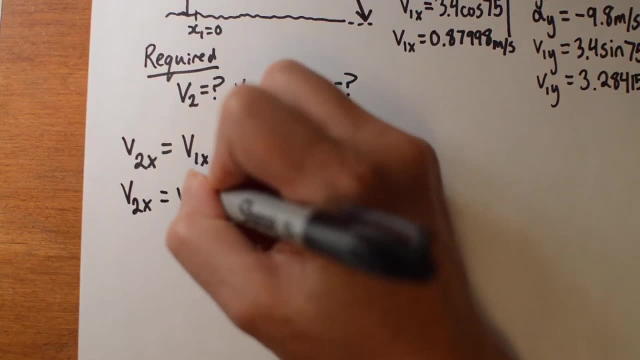 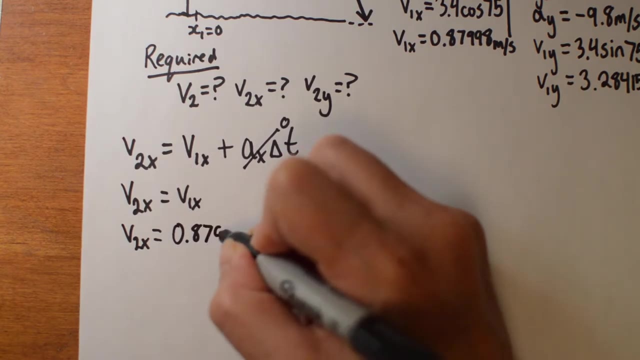 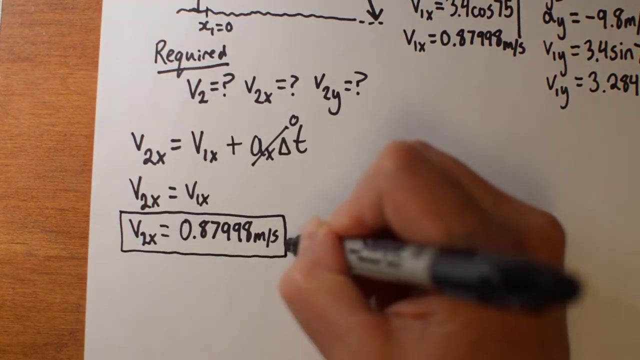 v2 is v1 plus a delta t, and just use the fact that ax is zero, right, then that term is gone and you just get that the final velocity is equal to the initial velocity. so i could write down the number there. v2x is 0.87998 meters per second. and there got it. i'm not done yet i need to put. 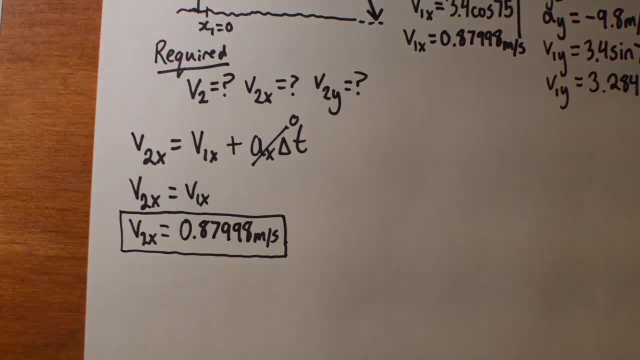 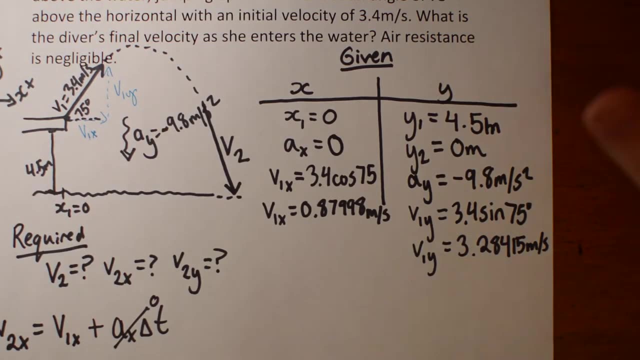 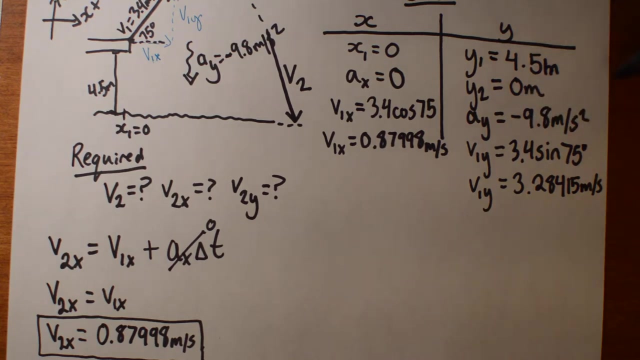 that together with v2y, but but there i have sort of half the bottle. it seems like- and i'm going to go back to what i know here and i can think about- well, which kinematics equation would really help me out here- and it looks like i don't have time right- so probably the first or second kinematics. 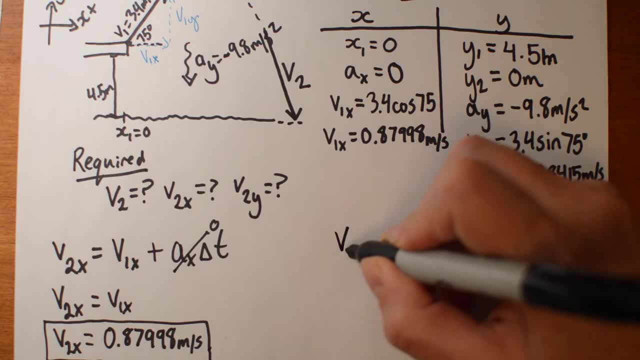 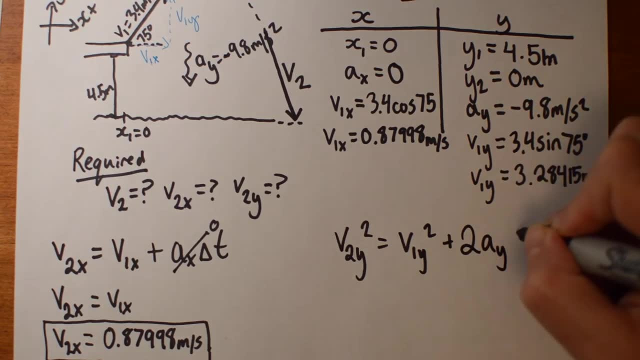 equations aren't good choices. but the third one is that v2y squared is v1y squared plus 2ay, y2 minus y1. this one is a really good one. i'm going to go back to what i know here and i'm going to 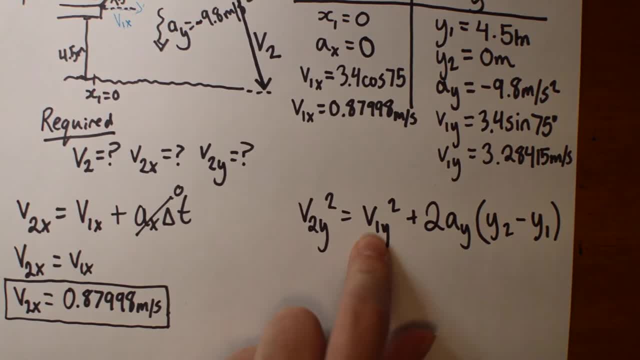 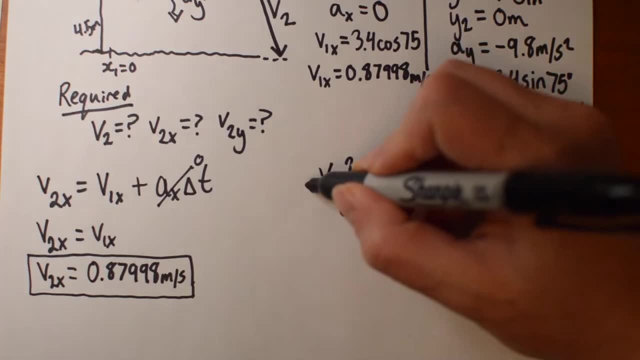 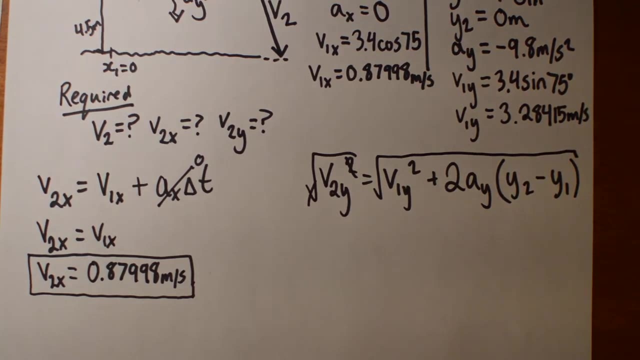 do a really nice equation because it has all stuff that i know right. i know v1y, i know ay, i know y2, i know i1 and it's even like basically rearranged for v2y. i just have to square root both sides, square that, that kills the square root, square this whole side and i've got v2y on its own. so 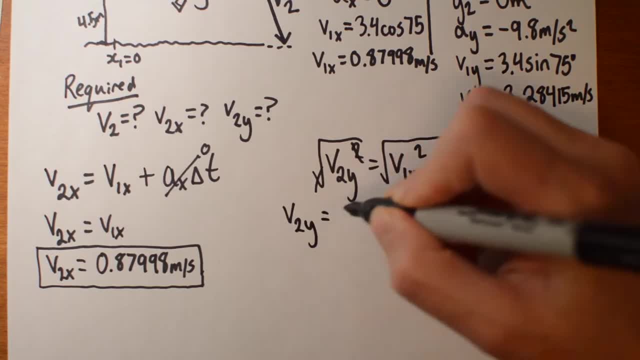 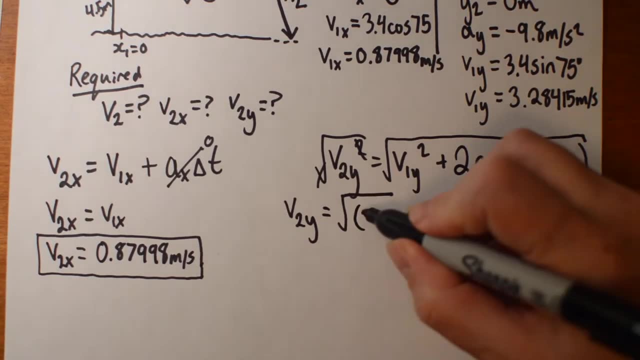 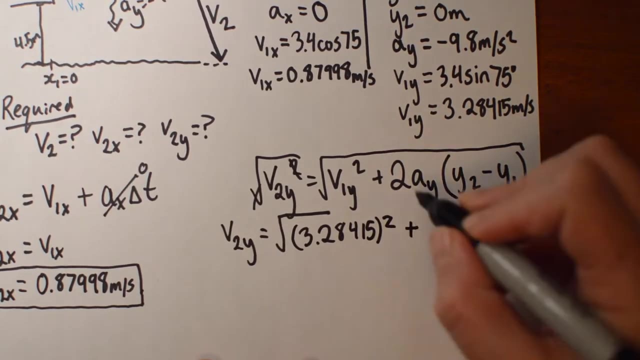 now all i need to do is plug in my numbers. so v2y is going to be the square root of v1y, squared. so v1y is this guy, right here the 3.2, 8, 4, 1, 5 and that's squared. plus i keep my square root sign going here because right that square. 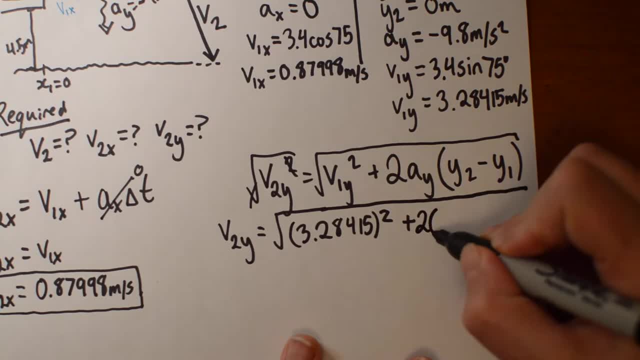 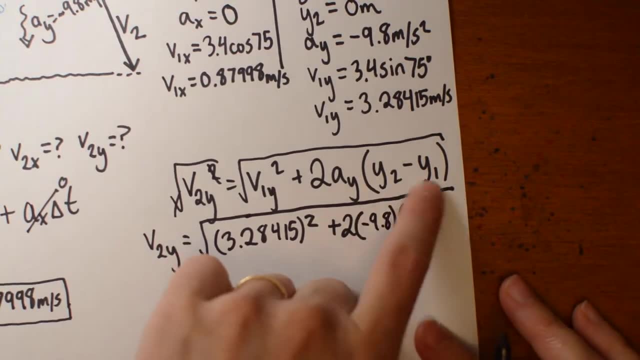 does not cancel that squared because it's adding in there. so 2 times ay, ay is negative 9.8. that negative sign really matters. y2 minus y1. it's important to get this order right too, because that's going to change the sign again. so 0 minus 4.5, so we're going to get like a negative times. 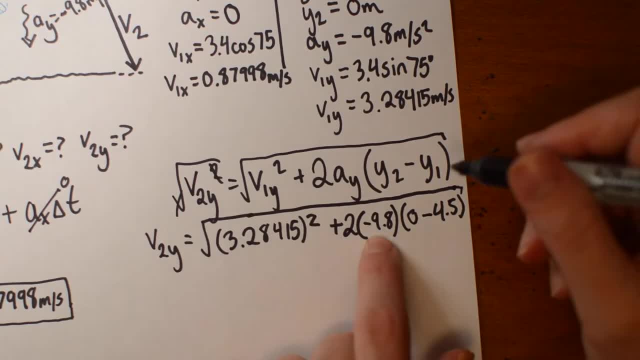 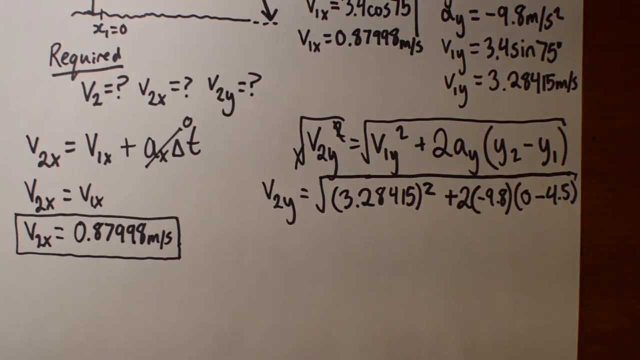 a negative, it'll make that whole term positive there, which is important, because that makes your v2y bigger than your v1y, which should make sense. you're sort of going down in this curve. you're further down than you were when you started, so you should be going faster. all right, we've got. 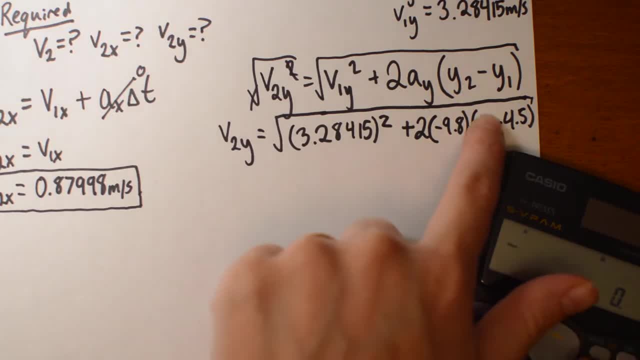 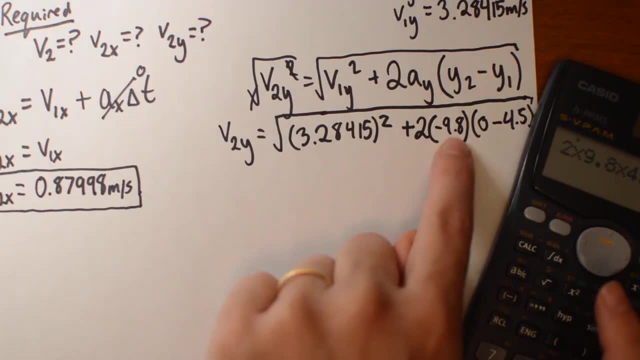 all our numbers in there, so we just need to toss that into a calculator. so i like to start with kind of this stuff in here. so 2 times 9.8 times 4.5, so i just sort of multiply those negatives in my head there. um, add that to this guy squared, so 3.28 415. 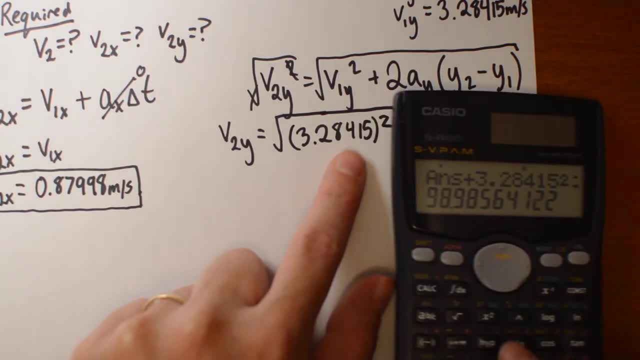 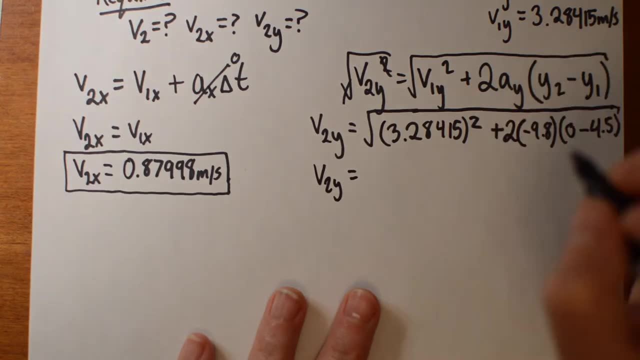 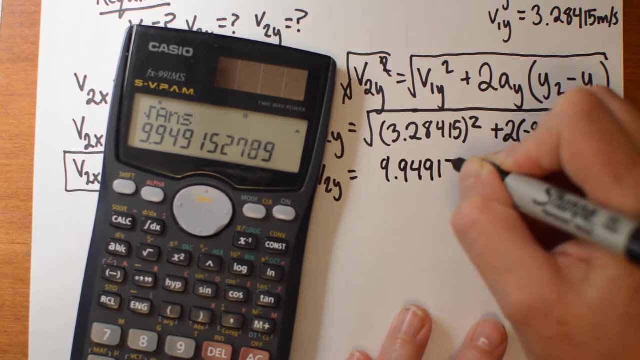 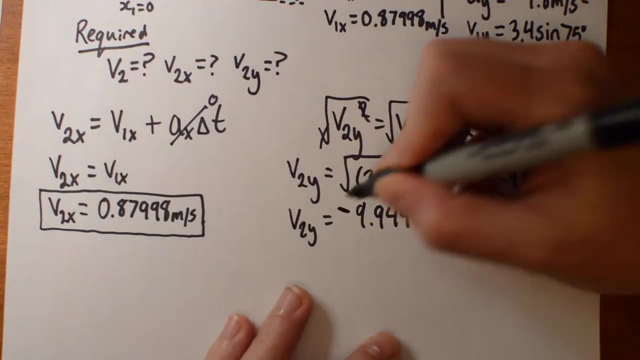 squared. so that's what's under my square root right here. square root, all of that and i get a v2y of plus or minus. right, this is plus or minus 9.94915 meters per second. and let's think about it from our picture. it's actually going to be a negative velocity, and that's because, in my picture, 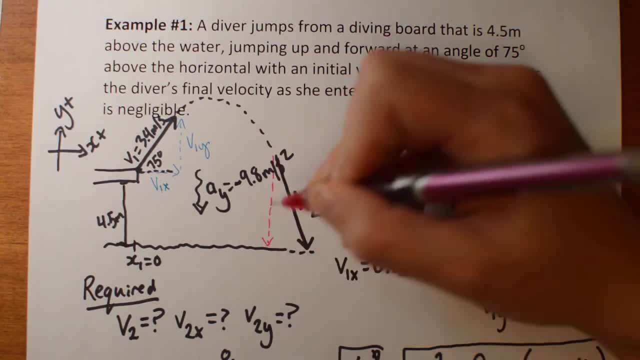 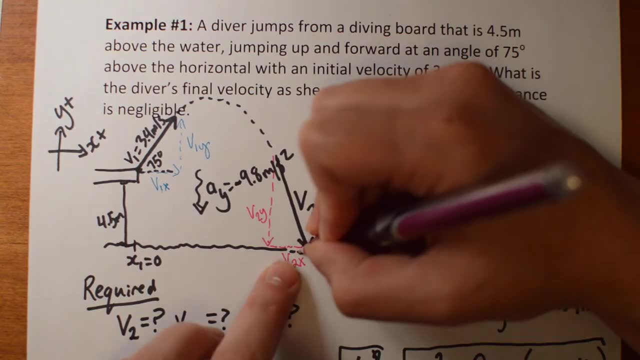 here i have two components to v2y and i have a negative velocity, and that's because in my picture v2 there's a v2y which is going down right and then v2x which is going forward. so v2x is clearly positive, this is going forward here, but v2y is negative, it's going down. so when you square root, 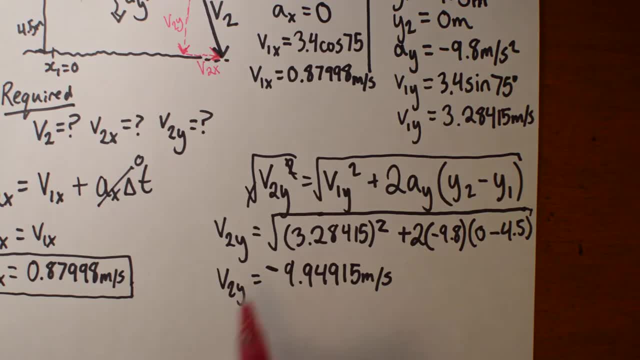 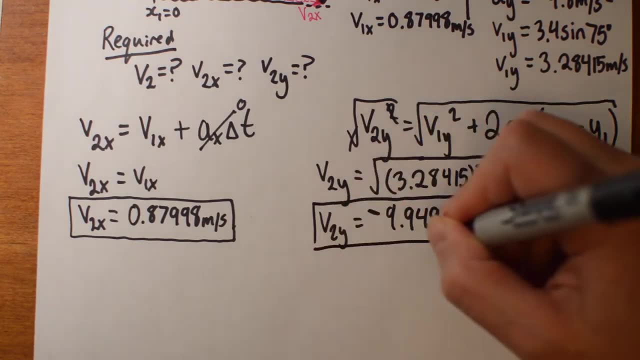 any number. you can get a positive or negative answer, but in this case the negative is the one that makes sense. all right, so i'm almost there. i have my v2x and my v2y. i just have to put them together to get the total final velocity. i like to do this in a little picture, so i'm going to 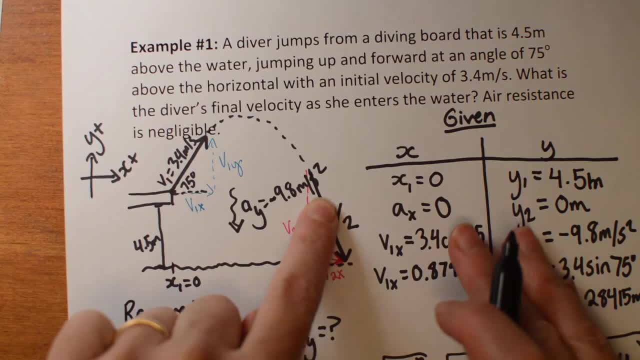 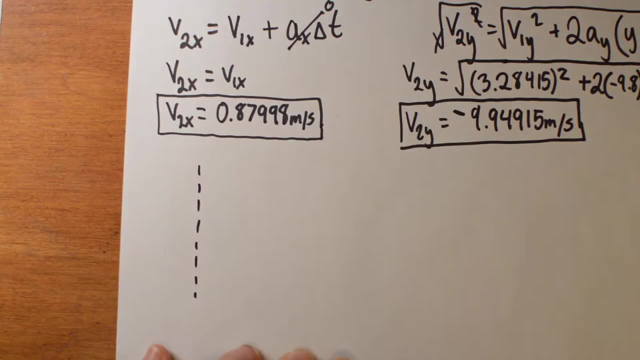 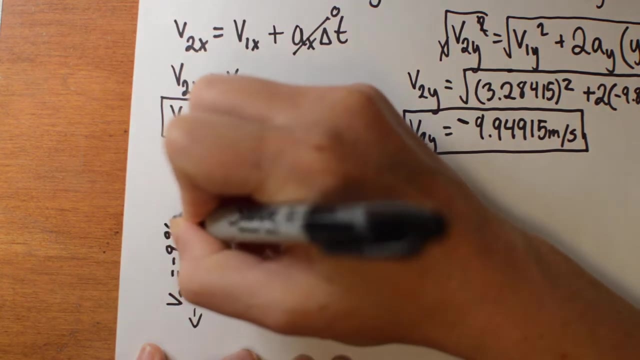 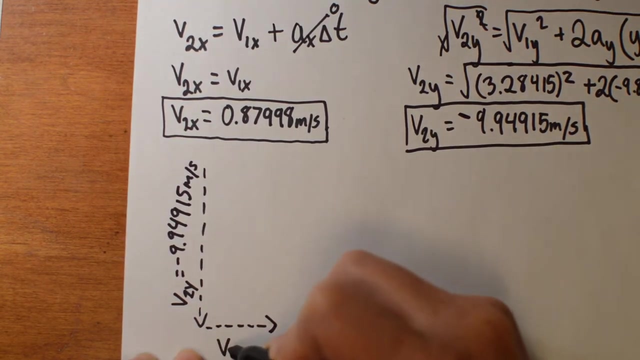 draw a little bit bigger down here. so i've got my v2y. here's v2y is the negative 9.94915 meters meters per second. and then i have my v2x is the 0.8409 meters per second. so i'm going to take this. picture here and sort of zoom in on it, draw it a little bit bigger down here. so i've got my v2y. here's v2y is the negative 9.94915 meters per second. and then i have my v2x is the 0.08925 meters per second. 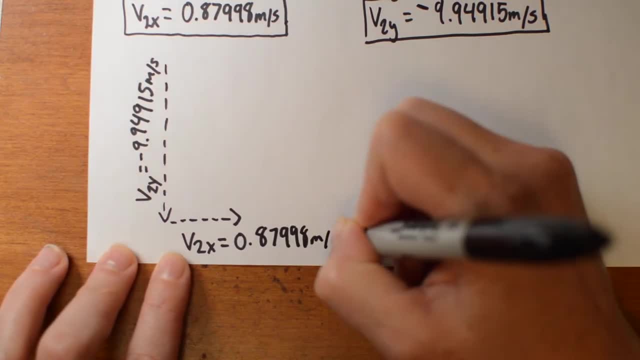 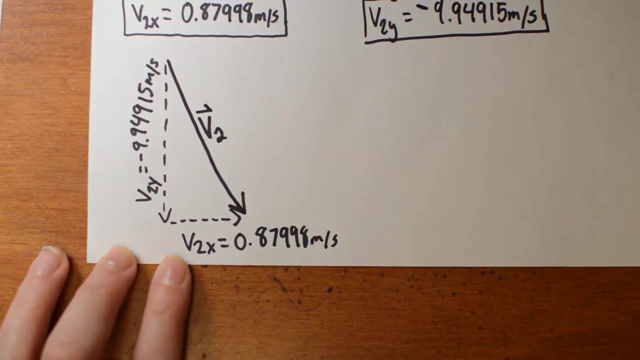 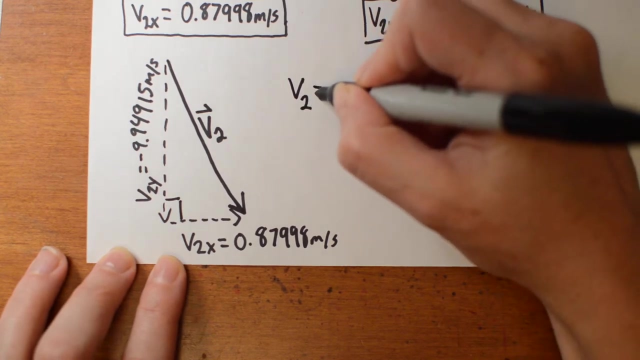 eight, seven, nine, nine, eight meters per second. and then i have the thing i want here, which is the v two, that overall vector. that's what i'm looking for. so first i'll use pythagoras's theorem to get v2, because this is a nice right angle triangle, right? so v2 is going to be the square root of v. 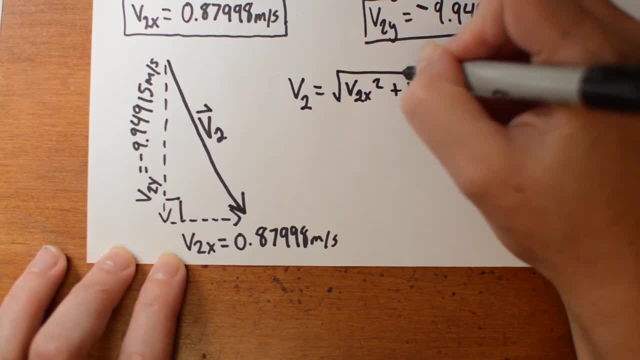 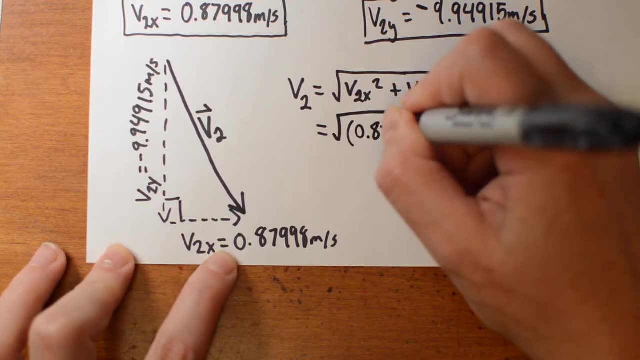 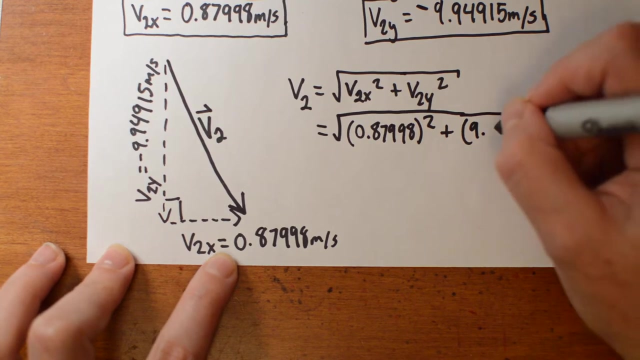 to x squared, plus v to y squared. that's just pythagoras's theorems. let's put in our numbers here. v2x is the point eight, seven, nine, nine, eight, that's squared. v2y is the nine point. it's negative here, um, but it's going to be squared, so it doesn't really matter. nine, four, nine, one, five, and that's. 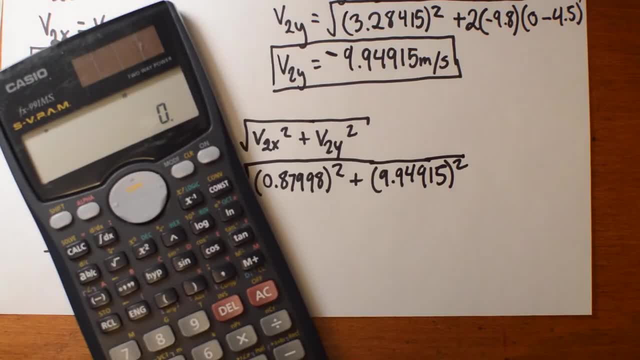 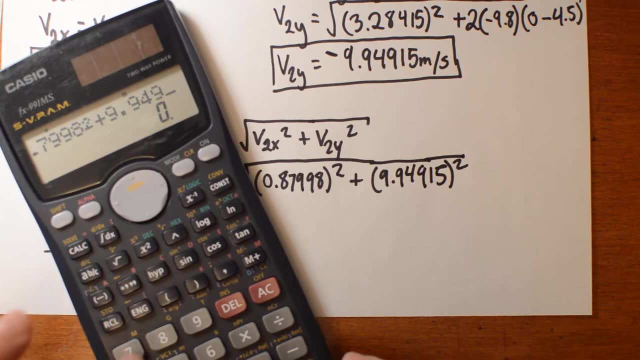 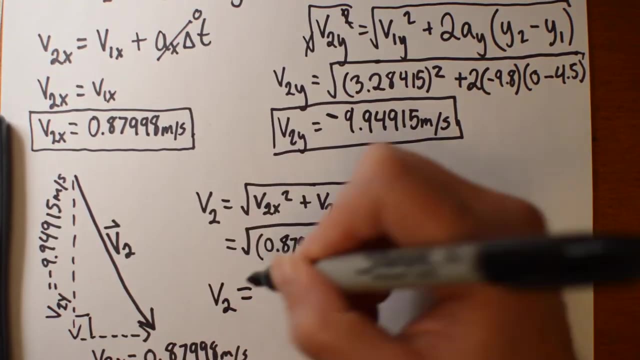 all right. so toss that into your calculator: point eight, seven, nine, nine, eight squared plus nine, point nine, four, nine, one, five squared and square root. all of that and i get v2. and here i'm going to round off to sig figs. so if you look back to your initial problem, 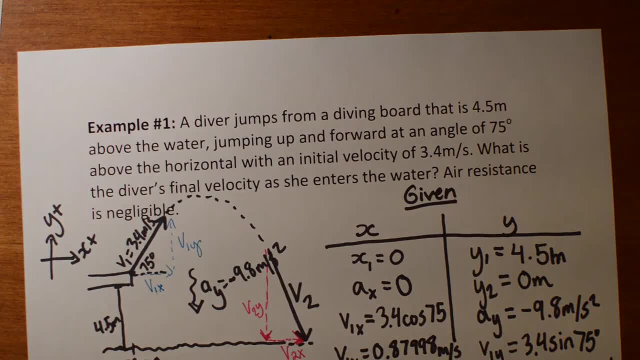 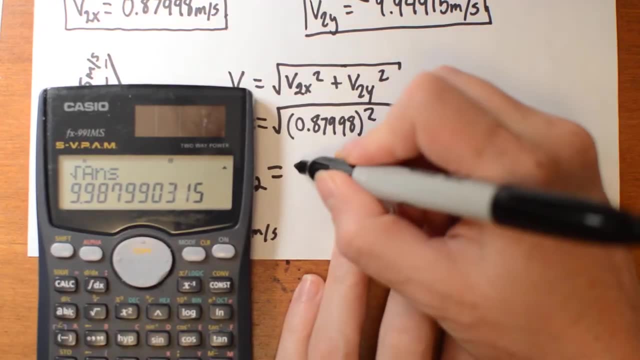 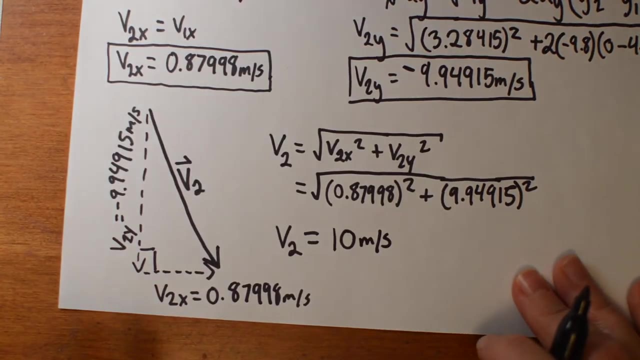 looks like i've got two sig figs. two sig figs. two sig figs, two significant figures, is the smallest number of significant figures, so i can round this off to nine point nine eight. we'll round off to just ten. right, just right on ten meters per second. it would be tempting to stop here, but i'm actually. 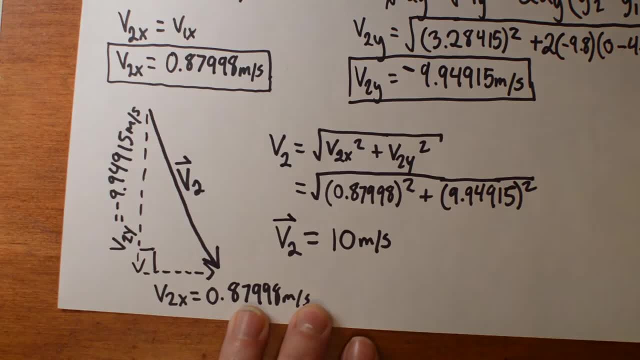 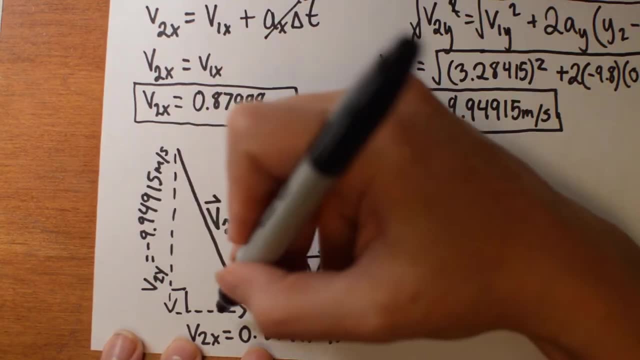 not done, because a vector- which v2 is a vector- requires a direction, so i can't just say off at some funny angle here. i have to say what that angle is. um, we could find either angle. i'm going to find this one in here, just because it doesn't matter, um, so i'll do that. 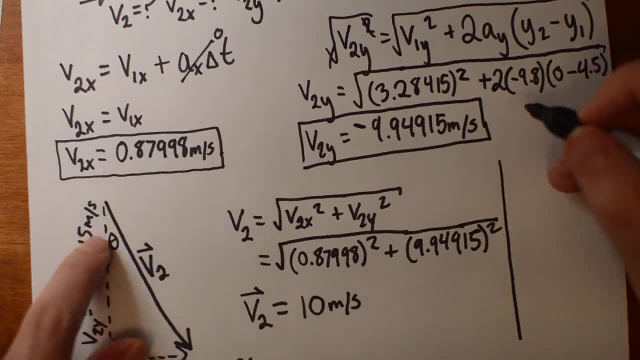 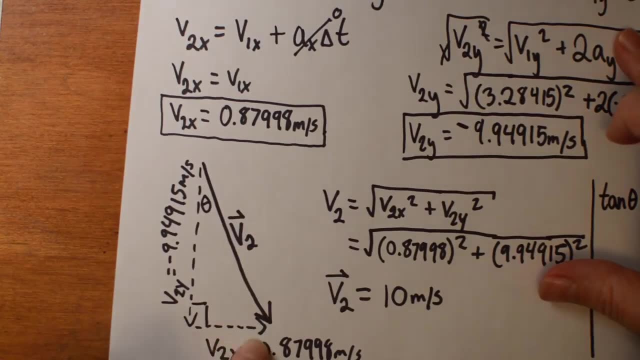 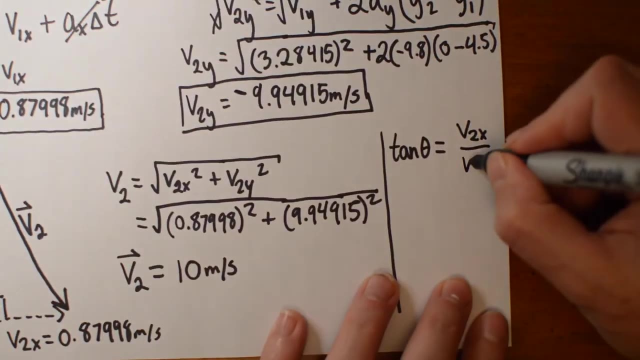 maybe on the side over here. um, that's going to be a nice toa thing of my sakatoa, so it'll be tan of my angle will be the opposite. the opposite is v2x divided by the adjacent, which is v2y. and if you remember when we talked about sakatoa, 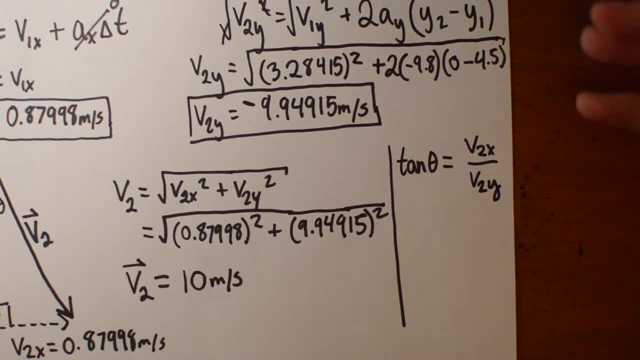 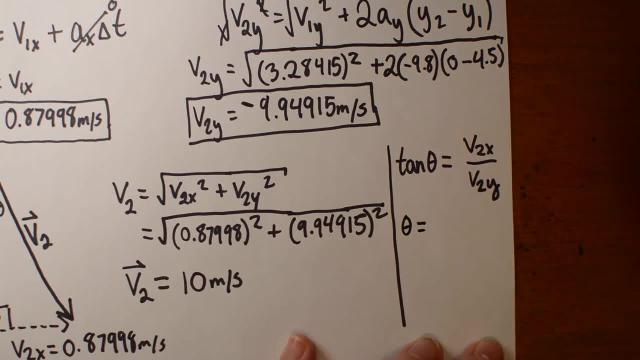 with these kinds of triangles, we don't have to worry about negatives or positives. if you do throw that in, you'll just get a negative angle, which is a weird thing to think of. so, um, you can put in the the positive number. that's fine. okay, i'm doing a tan function. i need an inverse tan tan to. 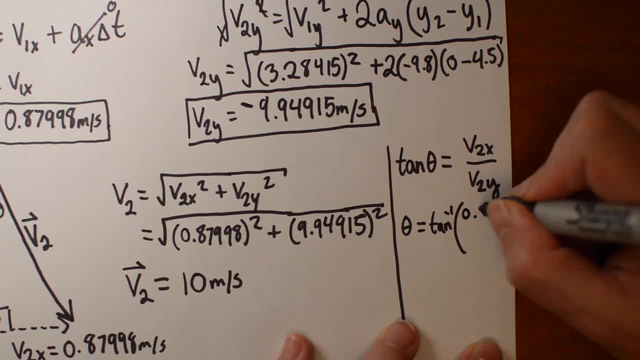 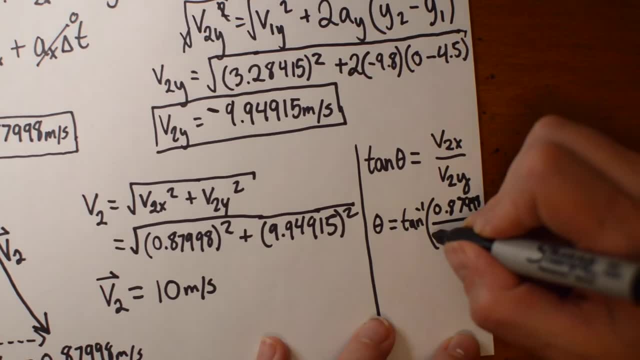 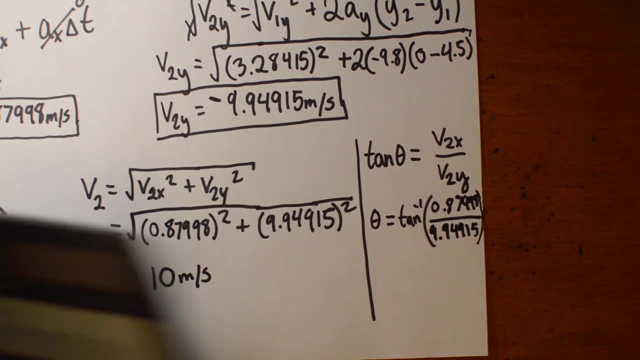 the minus one v2x on the top, that'll be point eight, seven, nine, nine, eight. on the bottom, v2y that's going to be the nine, point, nine, four, nine, one, five and i'll plug that into my calculator. so my v2x on the top, point eight, seven, nine, nine, eight. 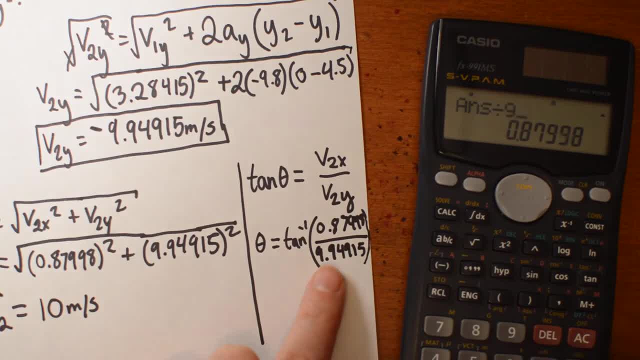 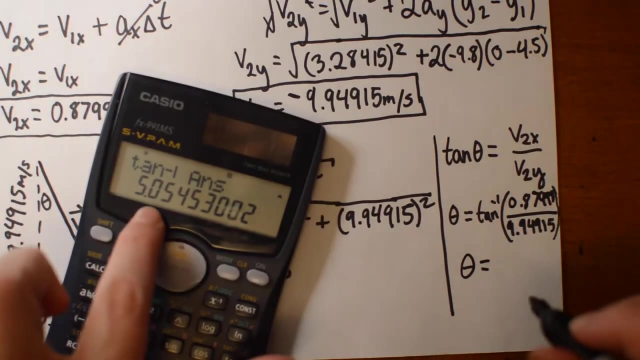 divided by my v2y on the bottom nine, point nine, four nine one five inverse tan that and i get five degrees in there. so pretty small angle, it's 5.05. so it's going to round up to 5.1 with my two degrees in there. 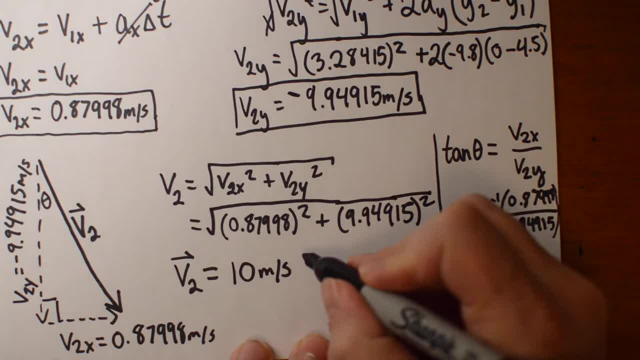 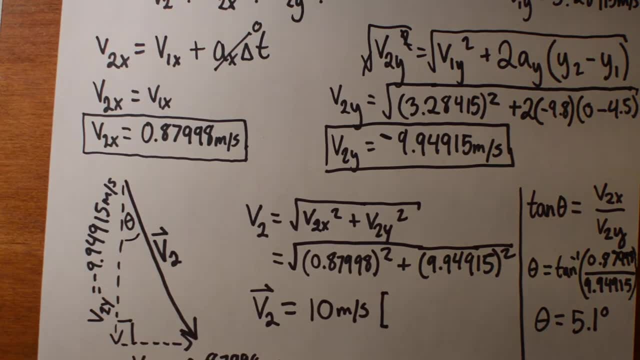 all right, so i can put a little square brackets here. it's best to just draw a picture and indicate where your theta is. that's good enough. you don't have to do more than that. but if you want to kind of describe it, you could say 5.1 degrees from the vertical. 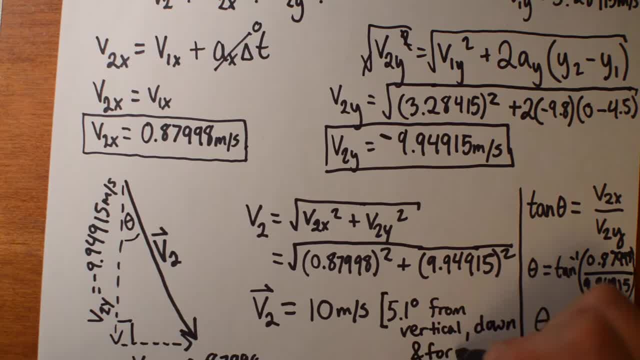 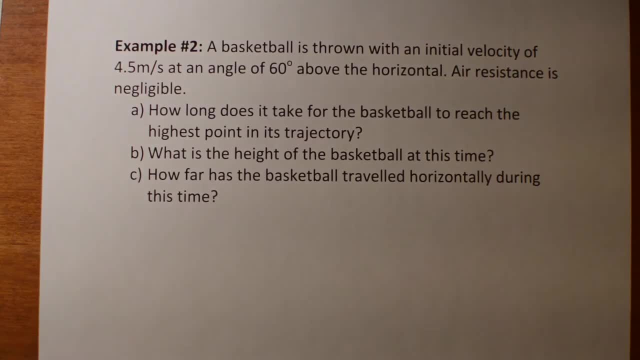 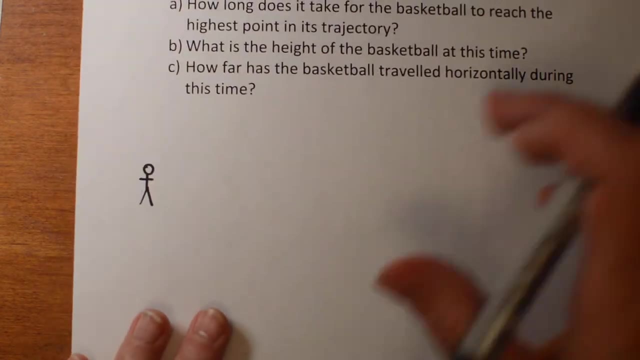 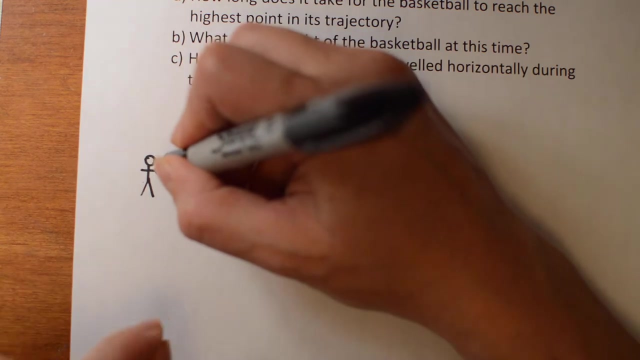 down and forward. you could say, and that is my v2 there. so in this example we have a person throwing a basketball. so here's maybe my person. here they're throwing a basketball from some initial height where it doesn't give us a height. so that means we get to set that height as zero. so we'll set sort of their hands as a y. 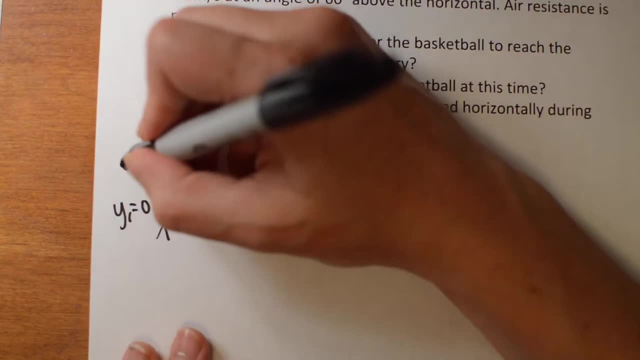 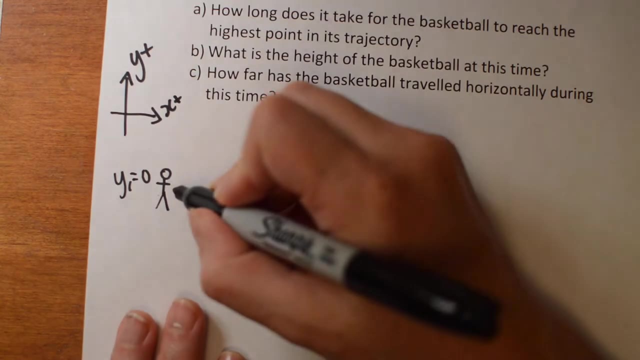 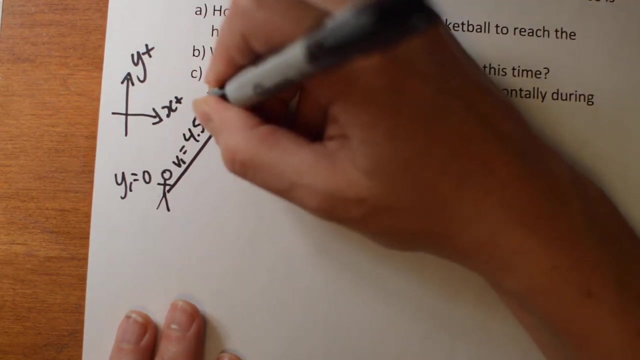 1 equals 0 there. we'll just put our coordinate system on here. so y is positive up, x is positive forwards. um, they throw it an angle, so it's going to be. there's a point. here is our initial v1, which is the 4.5 meters per second. the angle they throw this ball at is 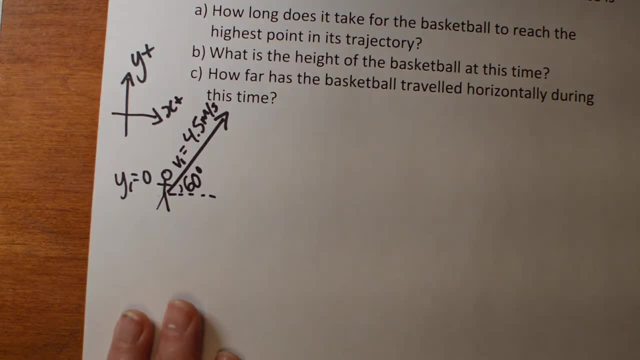 60 degrees here. um, air resistance is negligible, so the ball is going to do a trajectory like this right. what we're curious. curious about is that height, the highest point it reaches. we want to know how long it takes to get to that highest point. what that highest point? 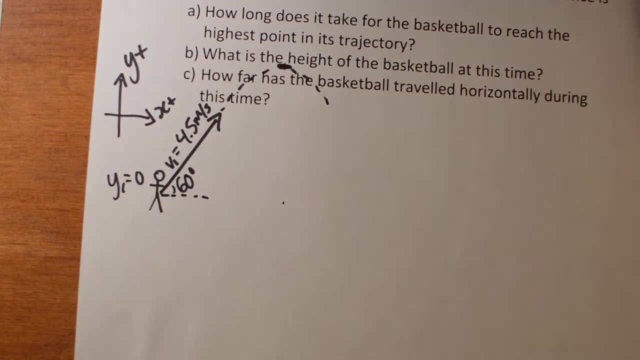 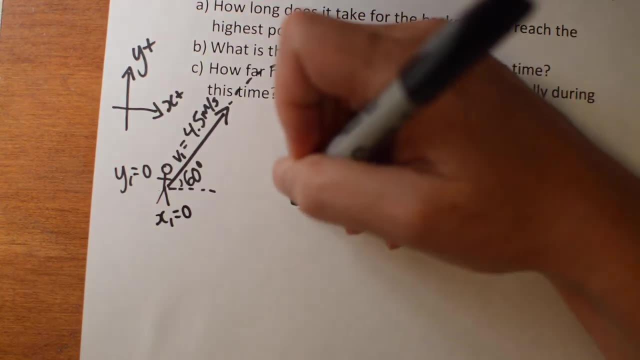 is and how far the basketball is traveled horizontally before reaching that point. so My x1 here will also be 0, and one of the things I'm looking for is going to be x2 at that point here. Alright, let's write down our given information. 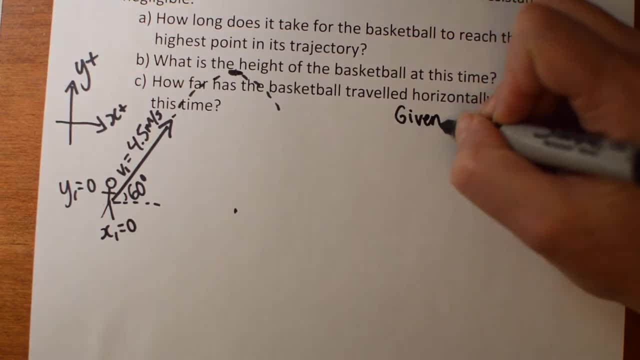 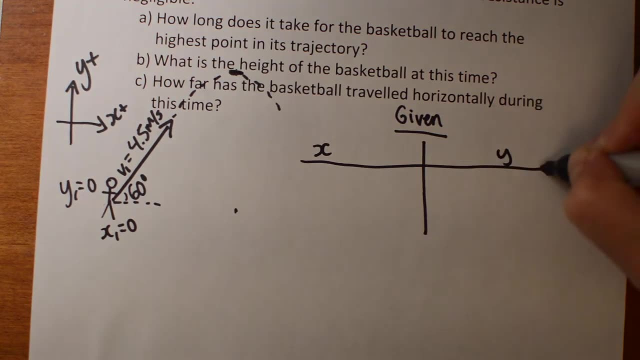 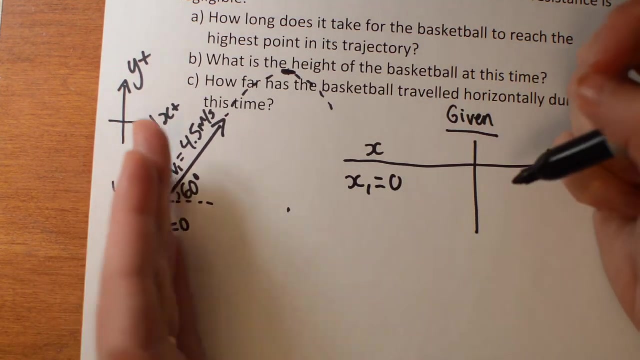 Always important to write it down as x and y separately. So I've got x here and I have y here. Okay, so x stuff. I know x1 is 0.. I started at no horizontal position and I'm going to gain some horizontal position as time goes on. 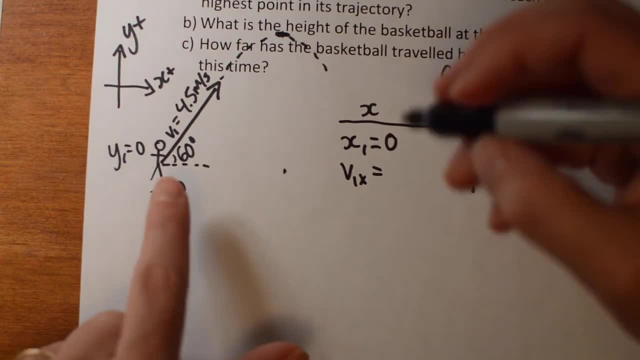 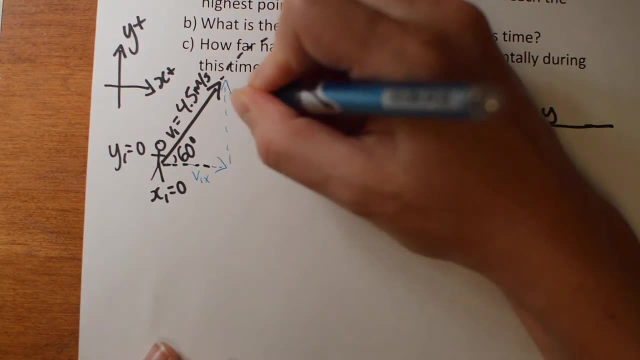 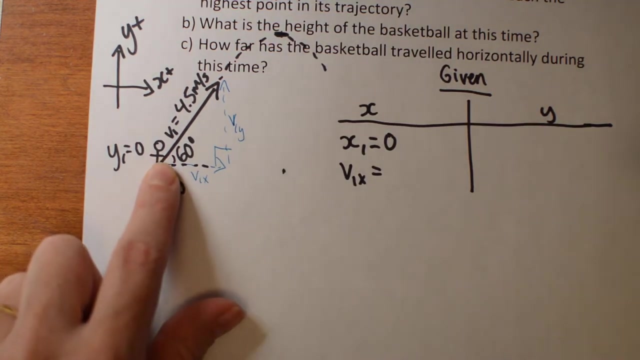 I know the v1x similar to last time. Just show us our components here. So there's a v1x here and a v1y there. That's a right angle triangle. v1x is close to the 60 degrees, so it's going to be cos. Cos is close. 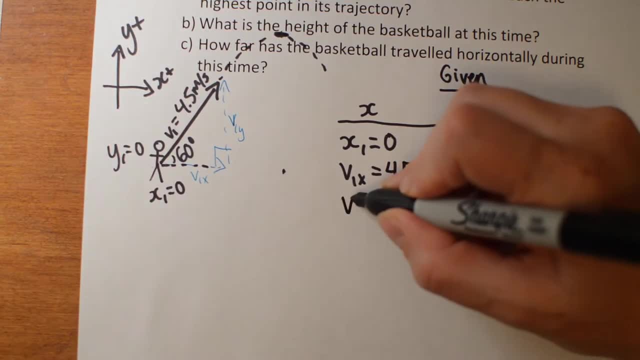 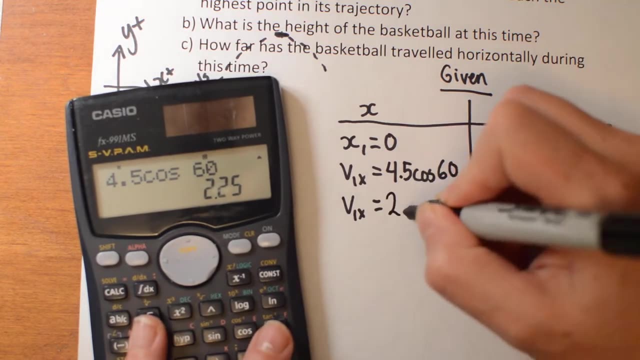 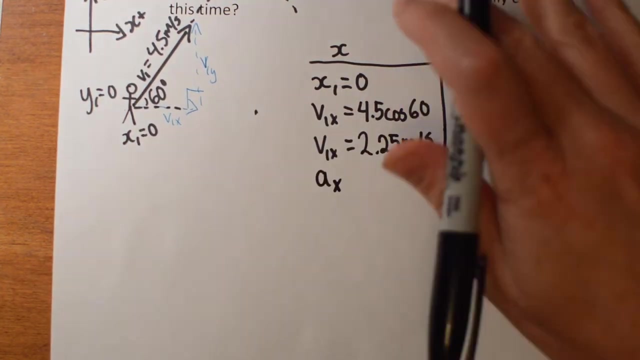 4.5 cos 60.. Let's get that, Let's get that number. So 4.5 cos 60 is 2.25 meters per second. The other thing I know in the x direction is the acceleration. So this ball is going to accelerate just downwards. 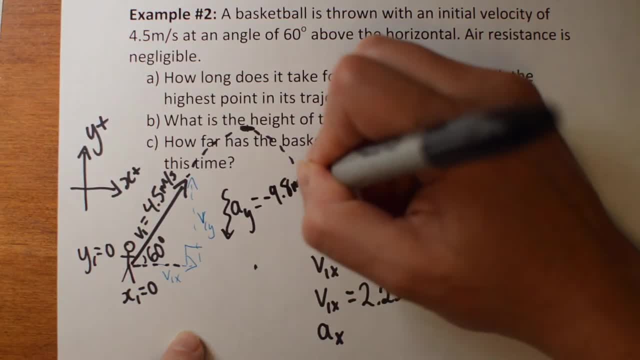 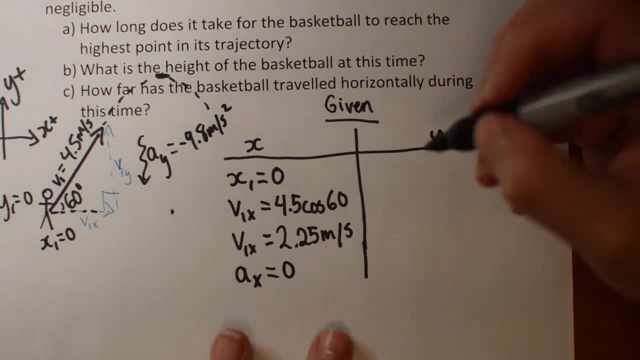 It's only going to feel gravity, An acceleration of negative 9.8 meters per second squared. It's not going to have any horizontal acceleration. so that is 0 there. Okay, in the y direction, Let's start out at a height of 0.. 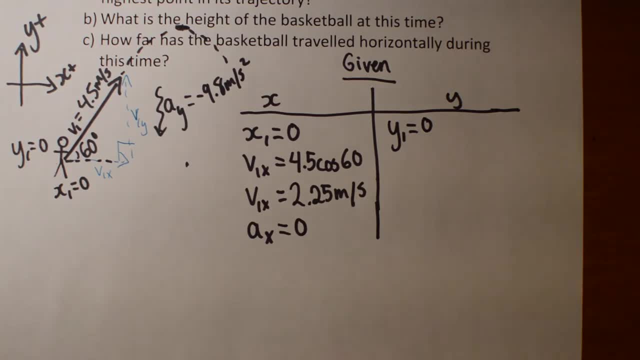 I mean, that's not really true for throwing a basketball. Your hands are usually not at the ground, But we can set our zero point anywhere, And because we're not given an initial height, that kind of works. We don't know what y2 is. 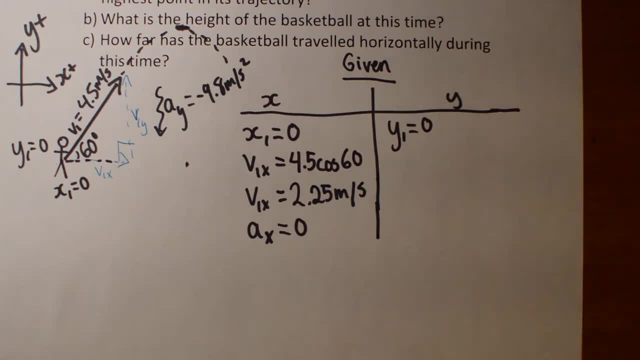 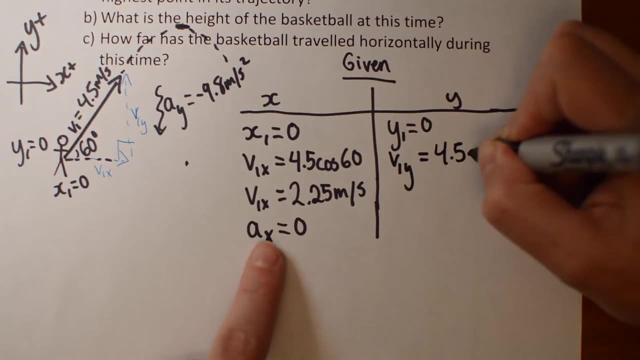 We don't know how high the basketball reaches in its whole trajectory. We do know v1y, though, Same idea as v1x. It's going to be 4.5 sin 60. Because v1y, you can see, is opposite the 60 degrees. 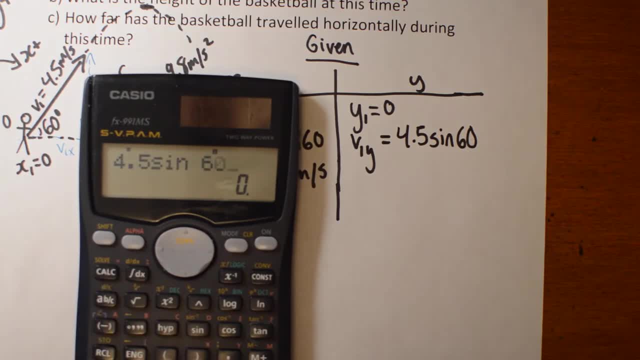 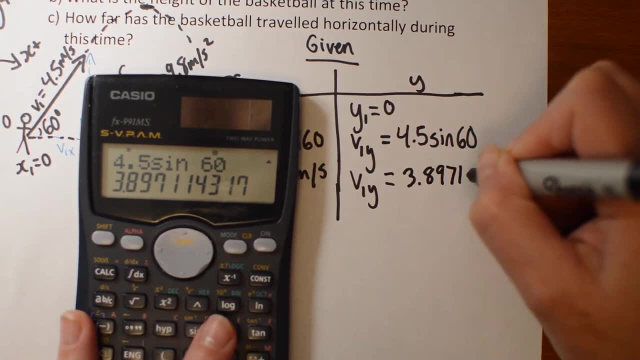 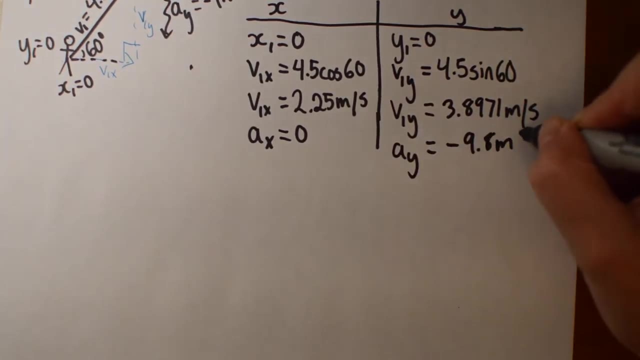 So 4.5 sin 60.. v1y is going to be 3.8971 meters per second And we know the acceleration in the y direction is negative: 9.8 meters per second squared. Okay. so our first question is all about time. 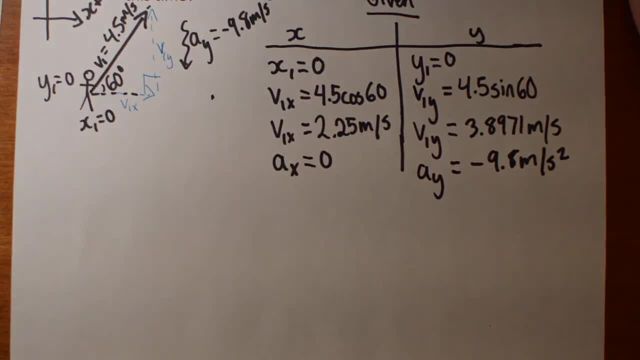 So we want to know how long does it take to reach the highest point in the trajectory? We look at all this information, It feels like we don't know enough stuff, And that's because I haven't written one really important thing down, which is how fast I'm going at the top of this trajectory. 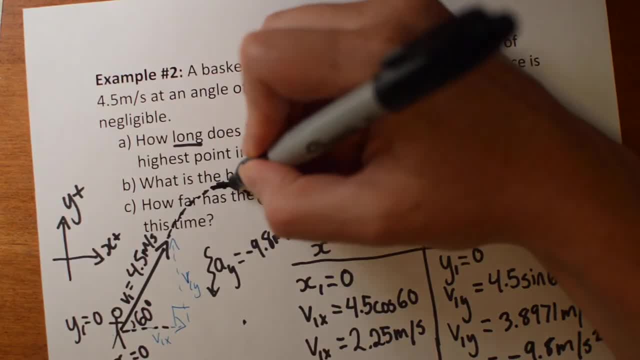 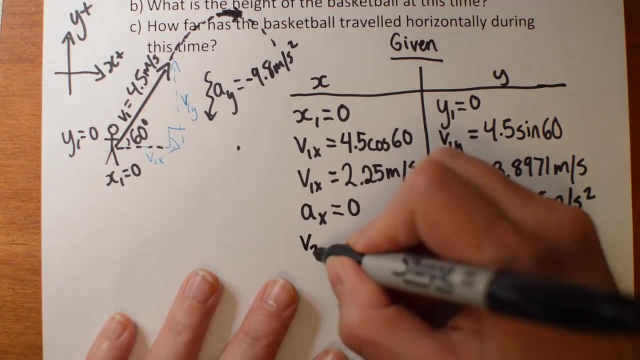 So when the ball goes through this whole trajectory, it's going to be moving perfectly horizontally at the top right. It's not going to be moving up or down at all. So its v2x is going to be just the same as the v1x. 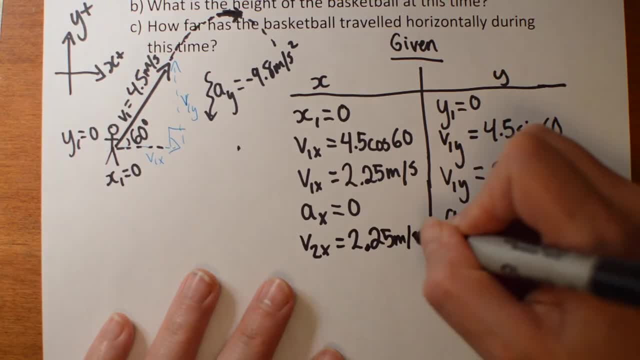 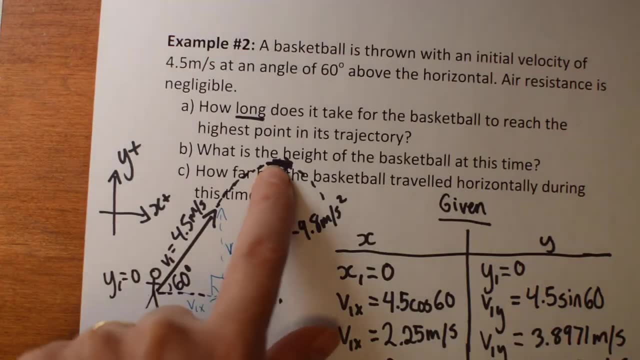 It'll still be bopping along at 2.25 meters per second, But its v2 in the y direction will be temporarily stopped, So it actually stops briefly at the top. It's going to be zero. That extra piece of information is enough to find out the time. 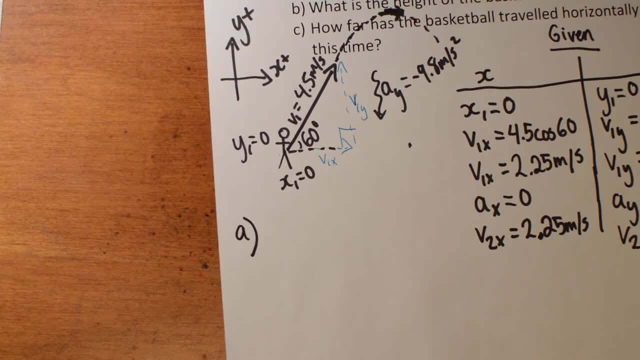 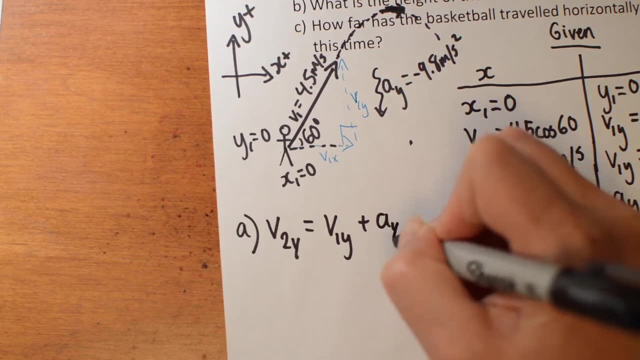 So I'll do a over here, finding time, And for that I'm going to use the very first kinematics equation, which is v2y is v1y plus ay delta t. So you see I know v2,, v1, a. 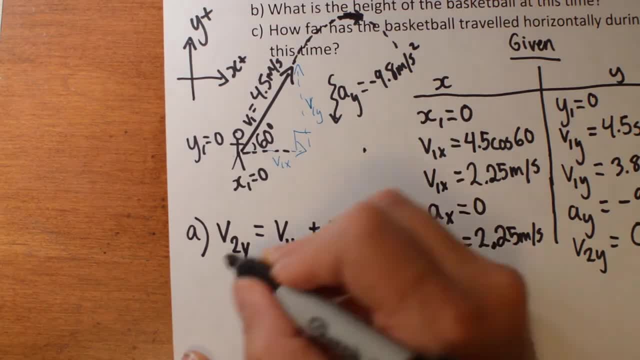 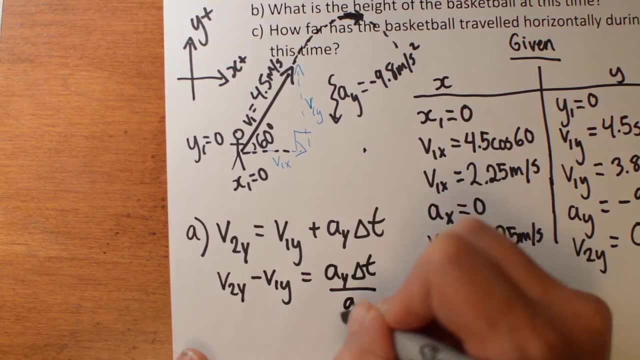 And all I have to do is find delta t. So rearranging that, put the v1 on the other side, v2y minus v1y, That's ay, delta t, And divide both sides by ay And we get delta t on its own. 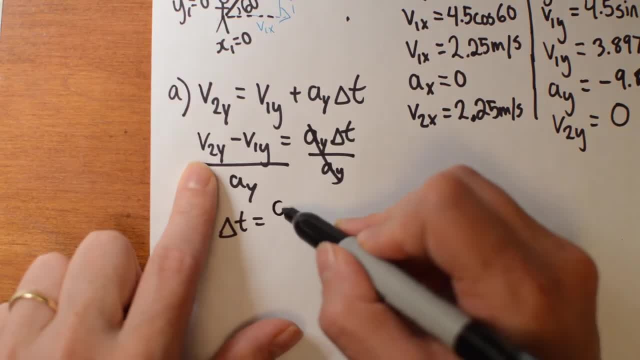 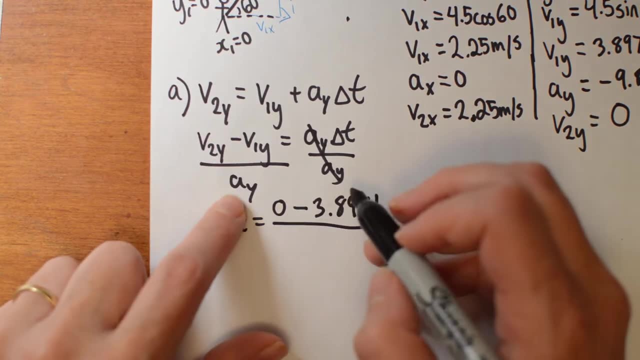 So let's calculate that delta t. Delta t is going to be v2y, that's zero minus v1y, which is the 3.8971, all divided by ay, which is negative 9.8.. I happen to have the v1y in my calculator. 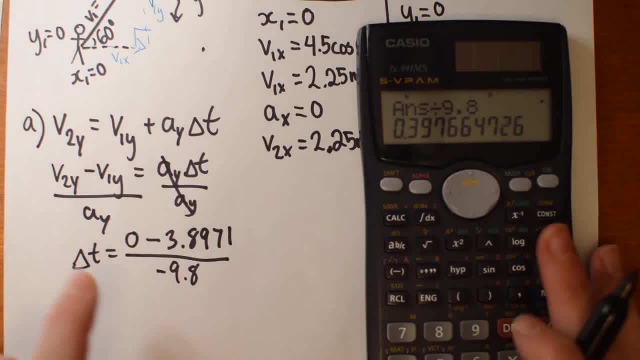 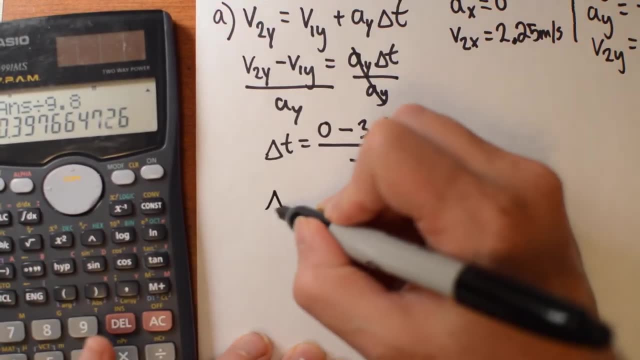 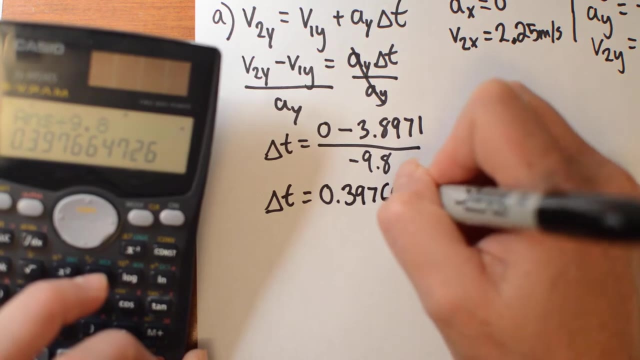 so I can just divide it by the 9.8.. Notice, I'm not worrying about the negative signs. There's a negative on the top, negative on the bottom, So we're going to make a positive when we divide those. So I get a delta t of 0.39766 seconds. 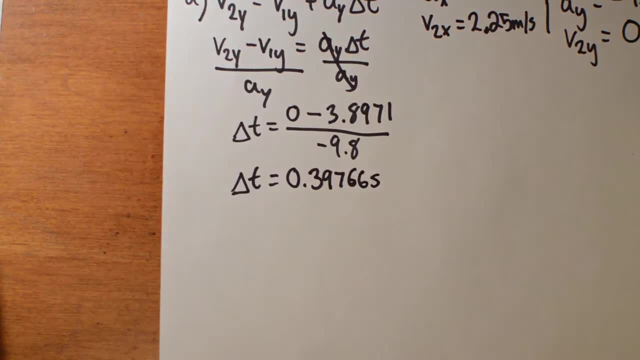 I'm writing down lots of decimal places right now Because this is like a part of the question. I have to also write it down in sig figs. But I'm going to keep all those decimal places in case I need the time for other things, which I will. 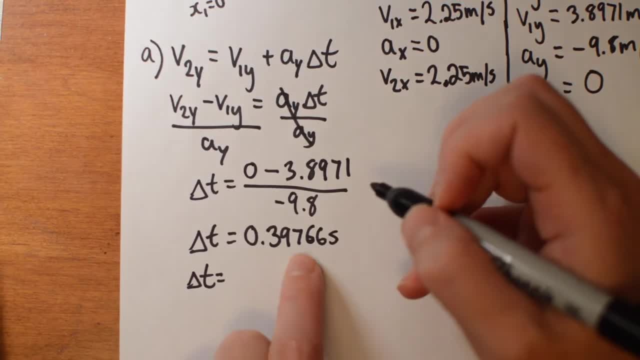 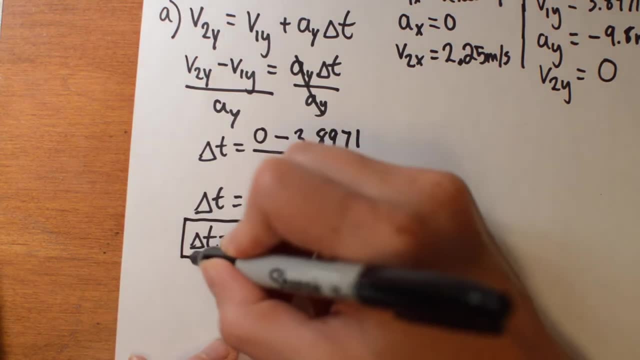 So now let's just write it down in sig figs, sort of round it off. That 7 is going to make that round up to a point 4, 0 seconds. So that's my time with the correct sig figs. 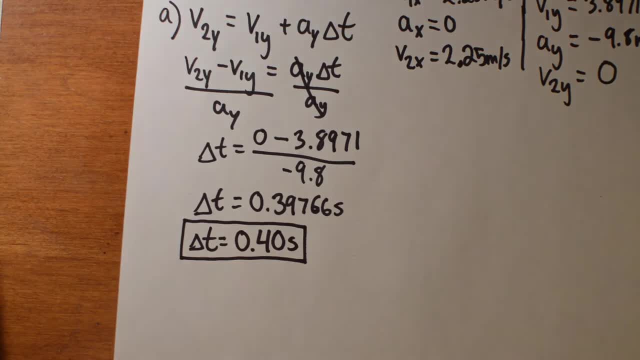 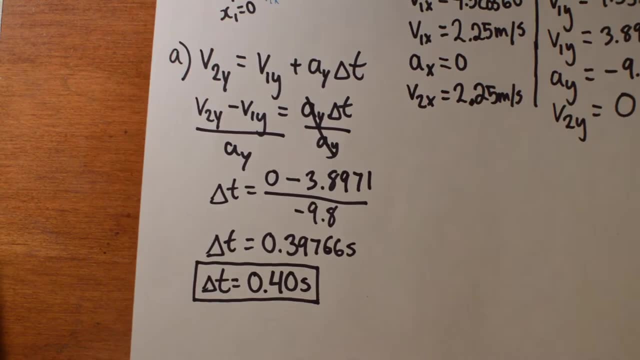 But I wouldn't want to carry that number through because that's going to have a ton of rounding errors on it. Alright, our next part is: what is the height of the basketball at that time? And that is actually pretty quick to find out, because the second kinemax equation is for y2.. 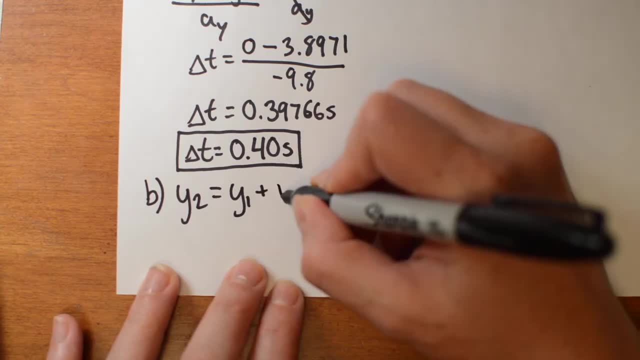 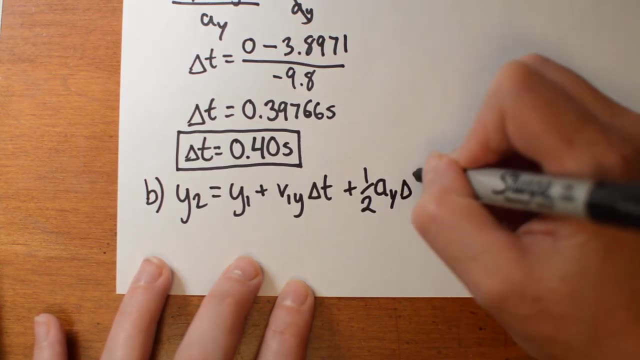 And it says y2 is y1 plus v1y a delta t plus a half a y delta t squared. So what's so great about this equation? it's already arranged for y2, which is what I need to find. 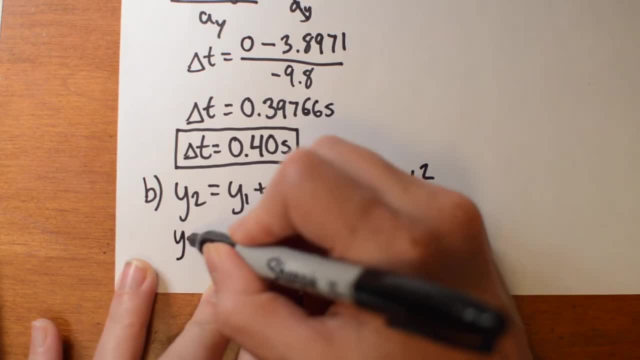 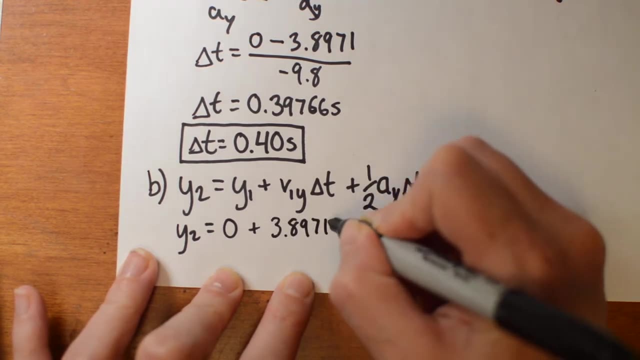 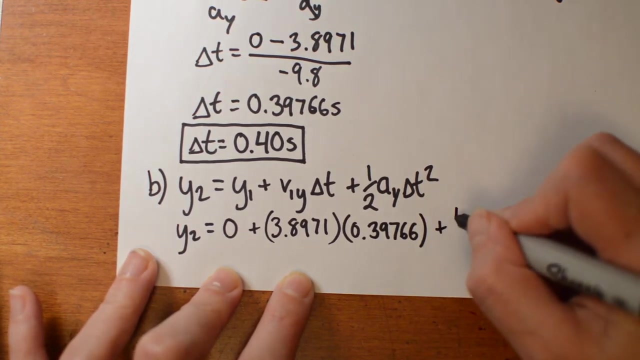 And we know everything in this equation. This is beautiful. So we just get to plug everything in. So y1 is 0.. v1y is 3.8971.. Delta t is 0.39766.. I've got my half here. 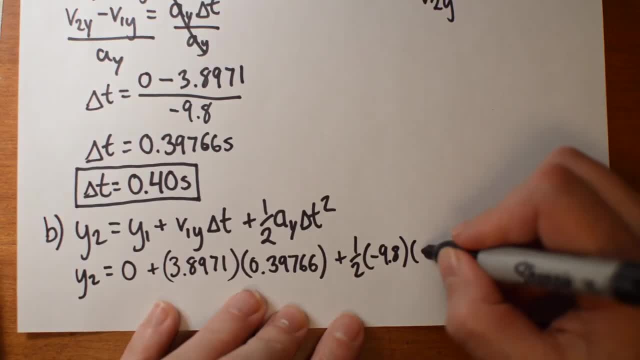 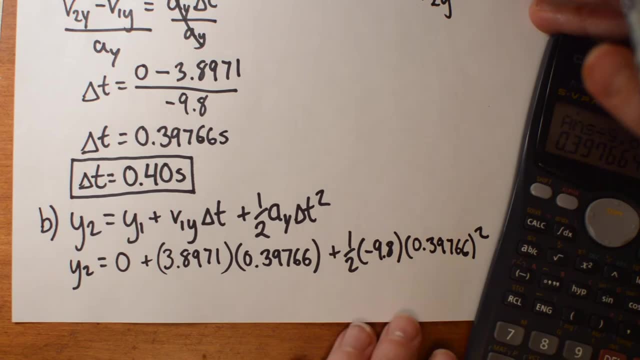 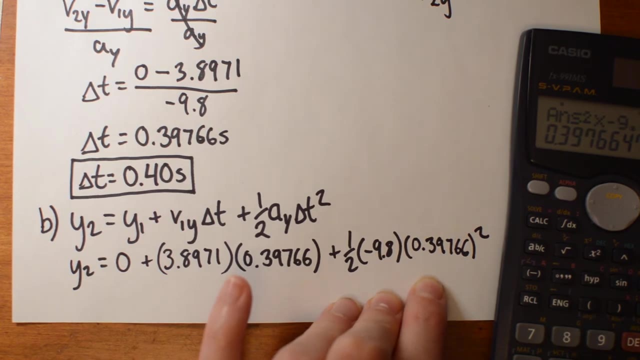 Negative 9.8 for a y. And I've got the time again. Times squared. Okay, toss all that into your calculator. I'll just work from the end here. So there's my times squared. times negative: 9.8 times a half. 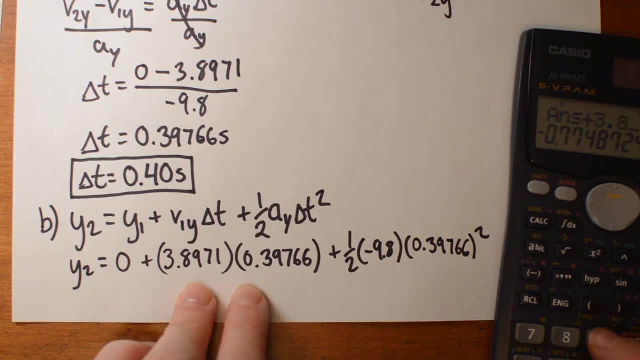 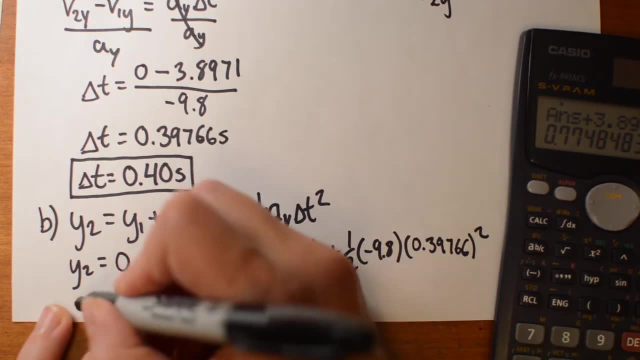 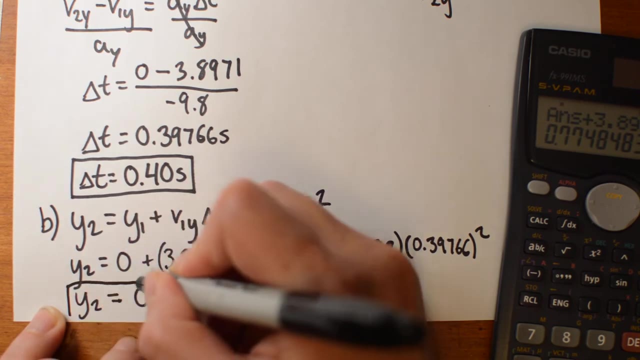 I'll add that to this next term: 3.8971 times 0.39766.. And I get a y2 of 0.77 meters. So this ball does not go super high in the air If you give a ball a small velocity. 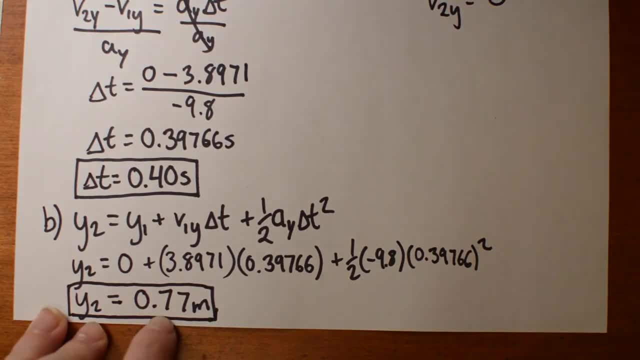 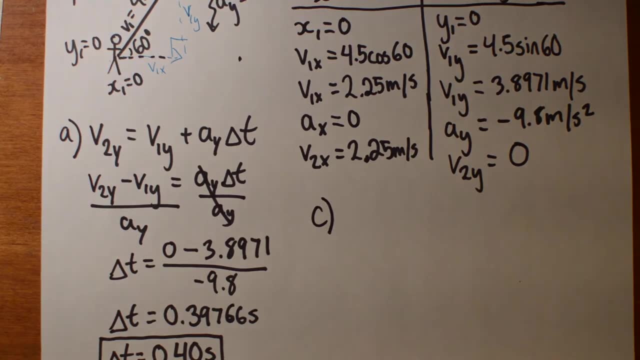 it's not going to go crazy high, So it just goes 0.77 meters in the air. Alright, last part, Part c, We want to know how far horizontally the ball has traveled in that time. We can actually use the same equation. 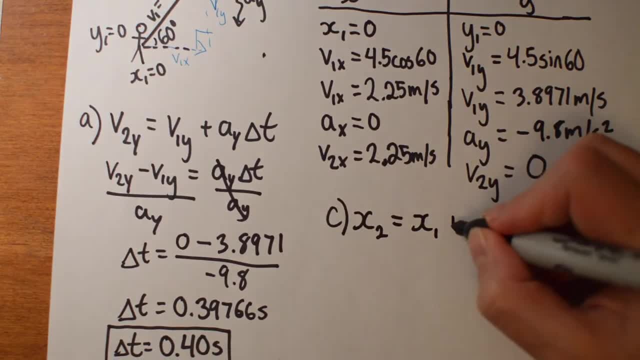 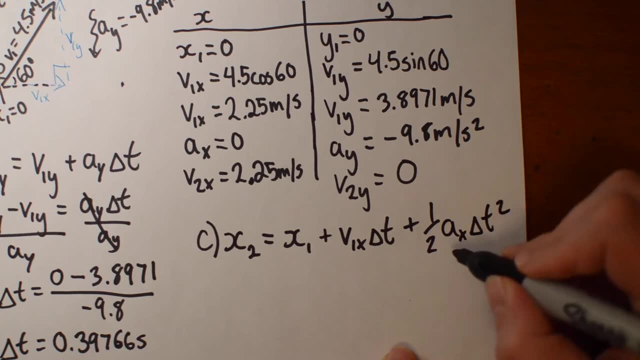 but for x. So x2 is x2.. Plus v1x delta t, Plus a half ax delta t squared. And this last term is 0 because it's not accelerating in the x direction- Ax is 0.. We also know x1 is 0.. 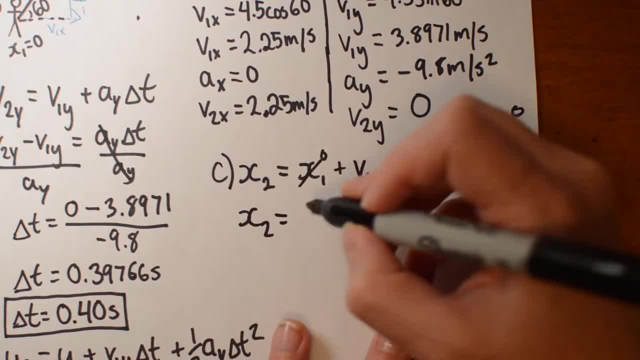 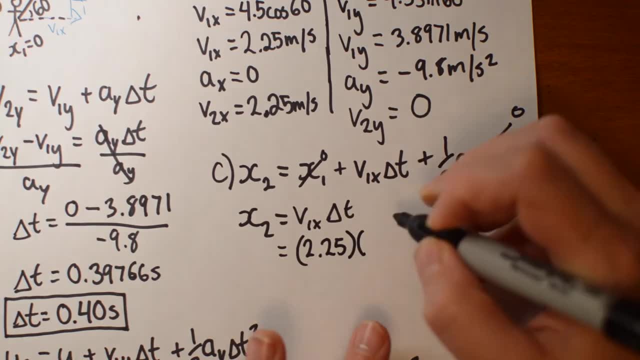 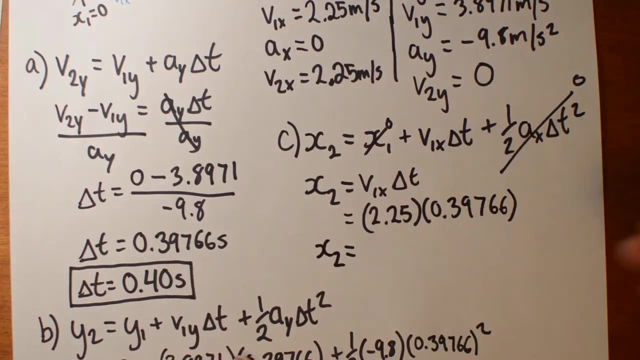 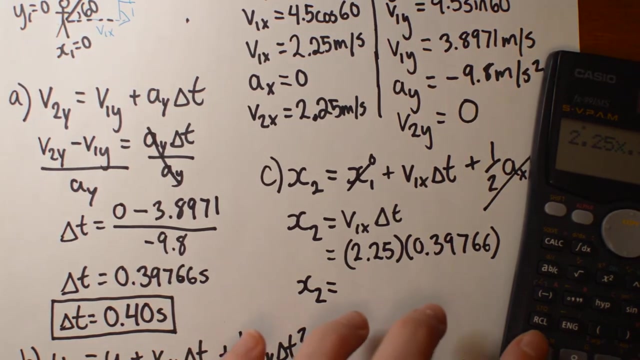 So this gets a lot easier. x2 is just v1x times delta t. Plugging in those numbers, v1x is 2.25.. Delta t is the 0.39766.. And I get an x2 of 2.25 times 0.39766.. 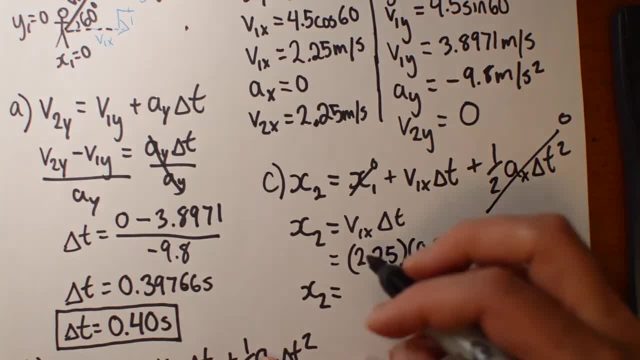 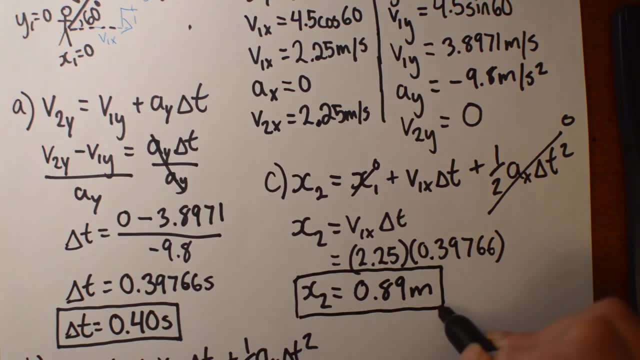 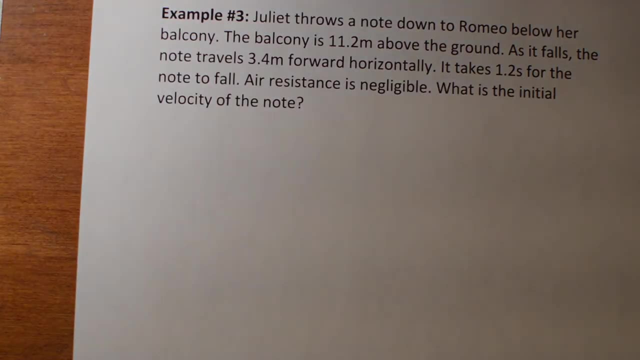 And I get an x2 of 0.89.. So it goes 0.89 meters forward And I'm done, Alright. our very last question: We've got Juliet up on a balcony and Romeo is below her, So the balcony is 11.2 meters above the ground. 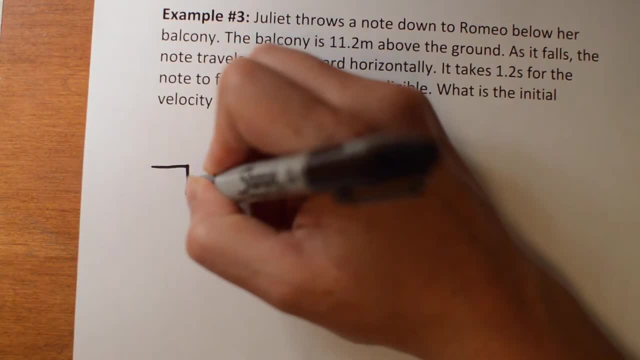 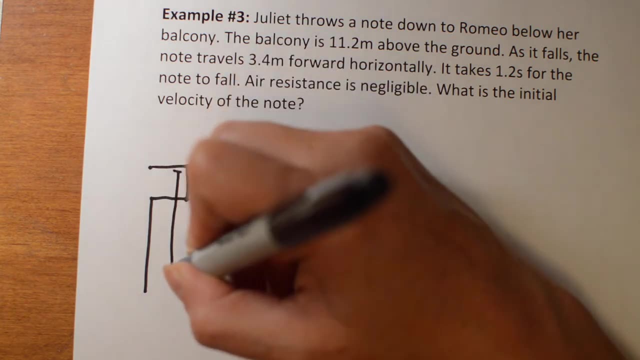 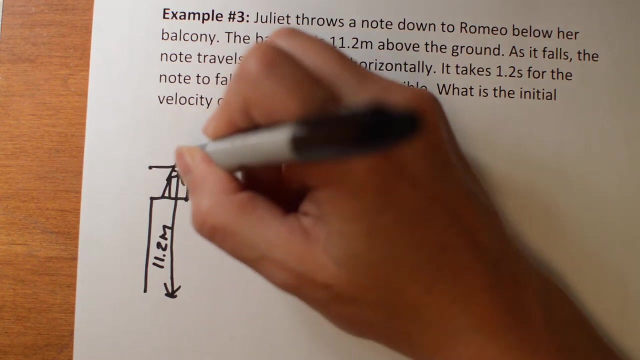 So let's kind of draw this here. Here's the balcony, So this here is this height from the top of the balcony to the ground. That is 11.2 meters here. So there's Juliet, She's leaning over the balcony. 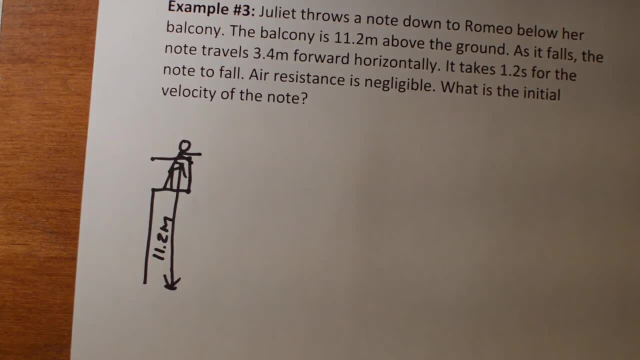 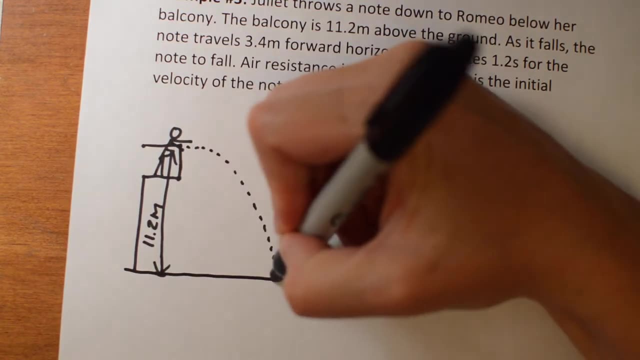 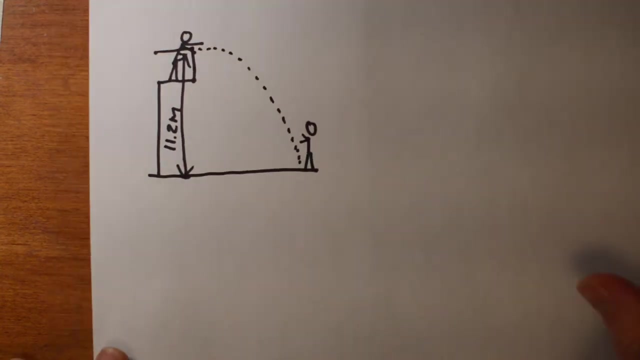 pining away for Romeo And she drops a note And we notice this note as it kind of falls. It sort of does some trajectory kind of like this: It lands on the ground by Romeo's feet And the horizontal distance it covers during that sort of fall. 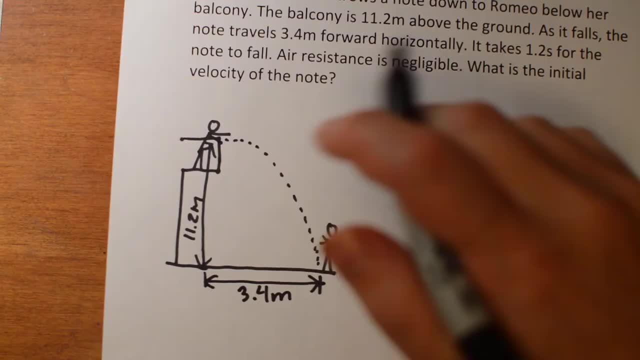 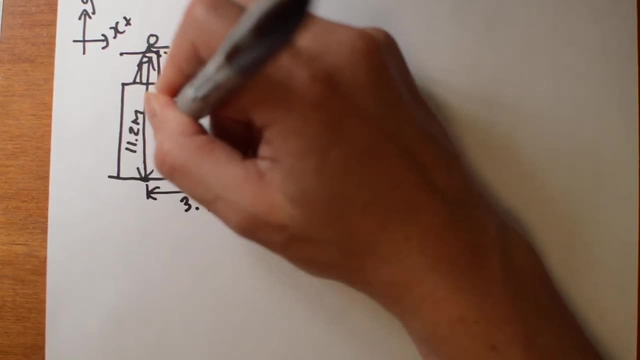 that distance right, there is 3.4 meters forward. Let's put a little coordinate system on here: y is positive up, x is positive forwards. This note is going to accelerate downwards at negative 9.8 meters per second squared. There's not going to be any air resistance. 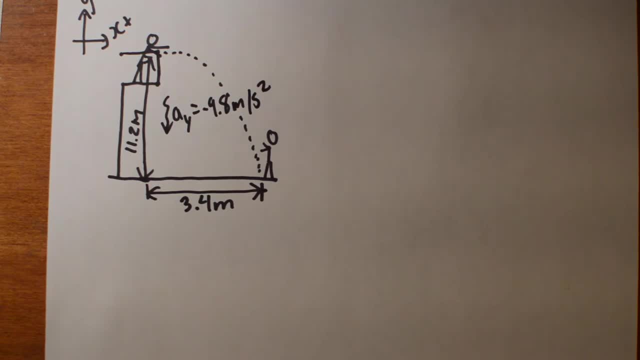 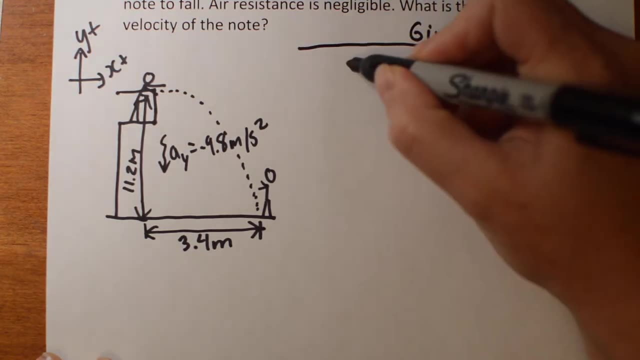 or anything messing that up. And we know it takes 1.2 seconds for it to fall. So let's write down everything we know, our given information. We know stuff in x, we know stuff in y, so we'll write it nice and separately here. 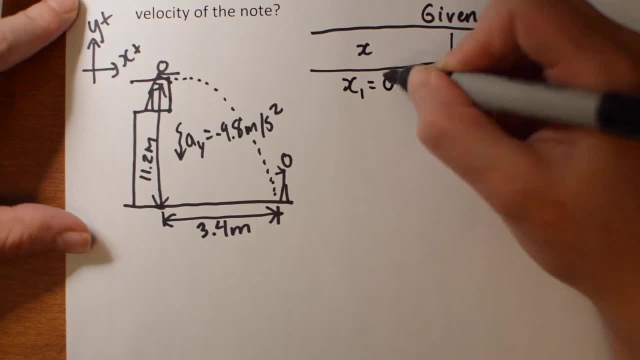 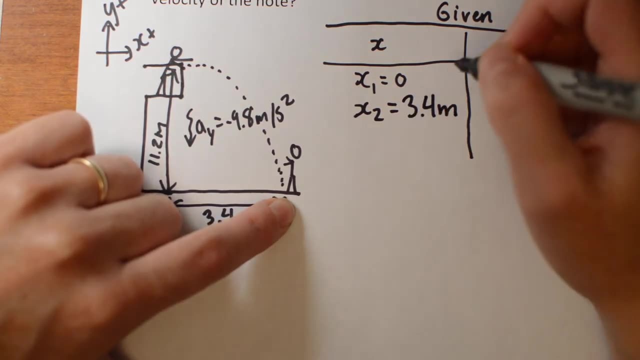 So in x, I know x1 is 0. The initial position of the note is 0. And after it's fallen it moves a horizontal position of 3.4 meters. Same idea with y right. I know y1 is 11.2 meters above the ground. 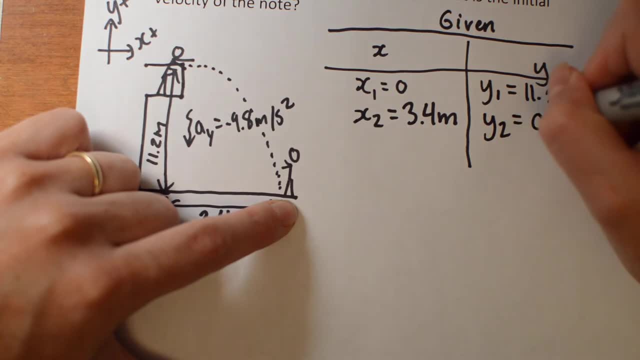 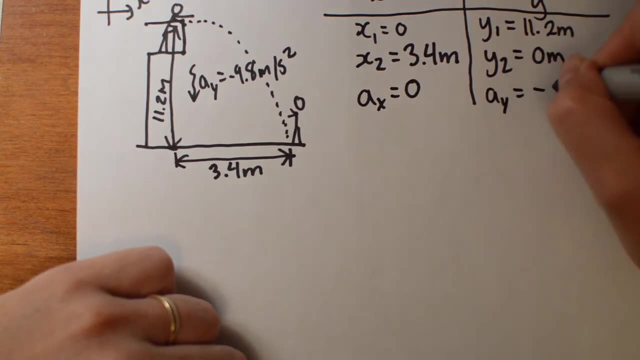 and by the time it's hit the ground well now it's at 0 meters. I know the acceleration, So ax is 0, and ay is negative 9.8 meters per second squared. The other thing that I know is the time. 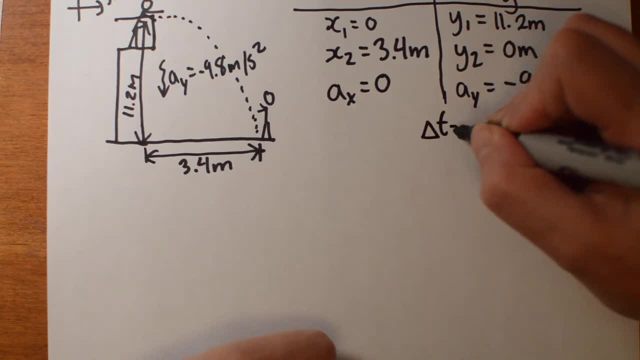 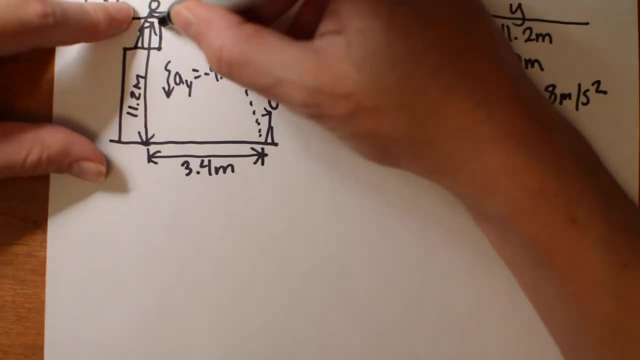 and that's kind of true for both. so I'll put it in between: Delta t is 1.2 seconds In this case. I don't know anything about the velocity. I don't know if she kind of throws it up initially. 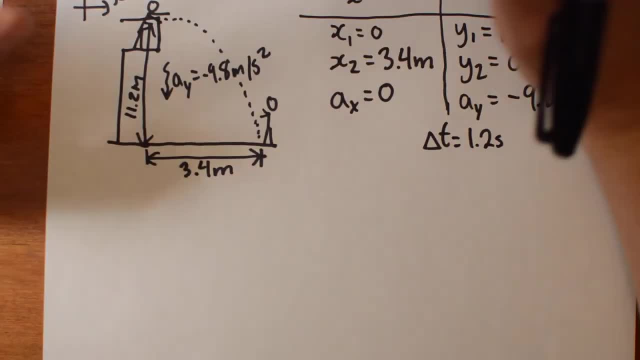 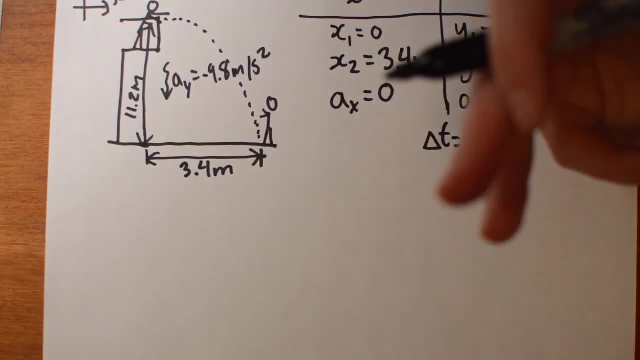 if she throws it kind of down, if she throws it perfectly horizontally. I really have no idea about any part of the velocity at all. So what I'm going to do is sort of work backwards from what I know to find out what that initial velocity must have been. 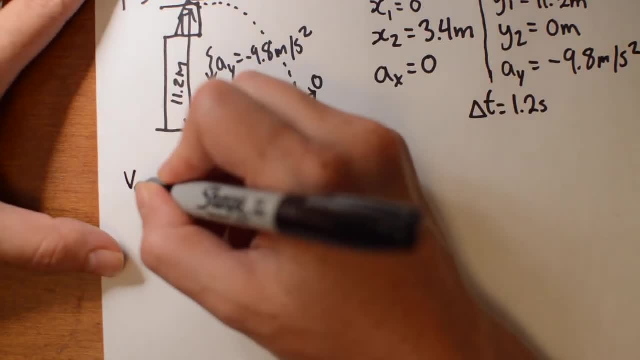 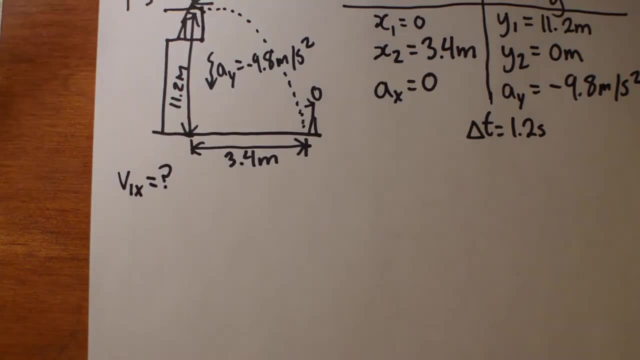 I'll start with the x direction to find out what v1x is. That's going to be my first goal. And then I'm going to find out what v1y is, find the vertical component and then I'll put that together to get the initial velocity. 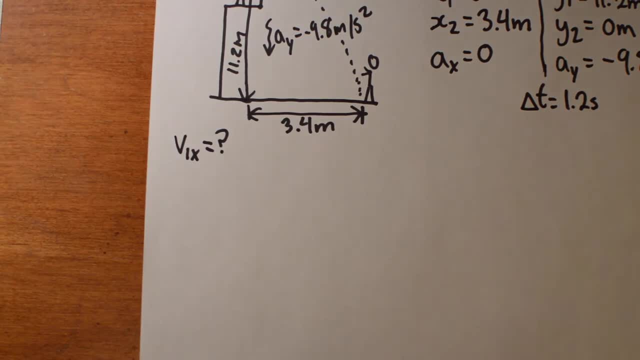 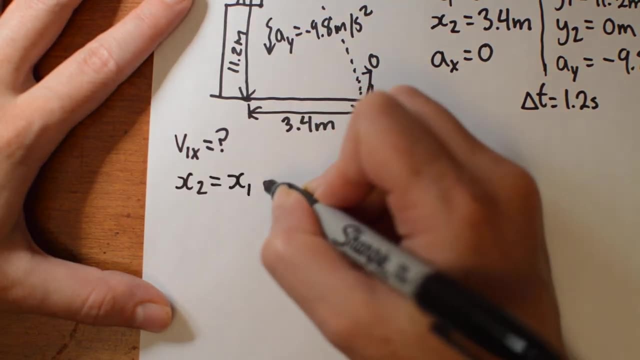 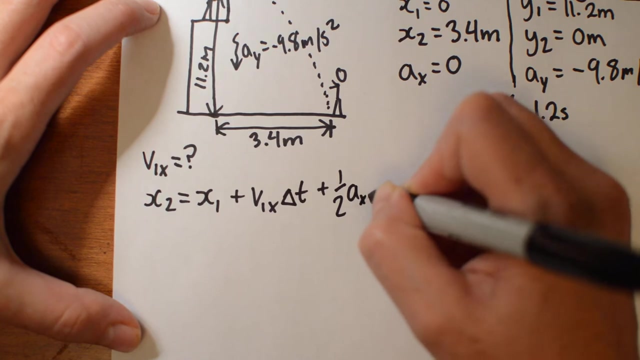 So first looking at the x direction, how about we use this equation here, So we could use your: x2 is x1 plus v1x delta t plus a half ax delta t squared. This is a nice equation, especially in this case. 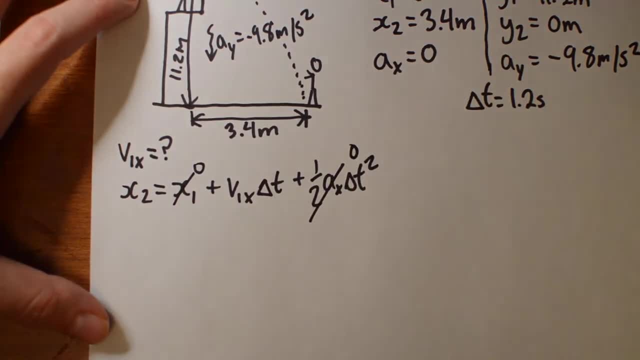 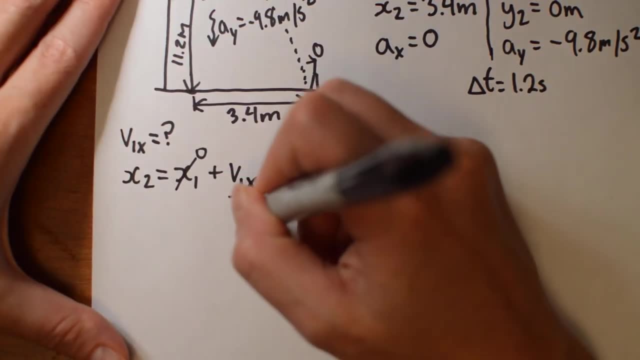 because x1 is 0 and ax is 0, so those terms are all gone. And then the next equation: x2 is v1x- delta t. I can rearrange that for v1x by dividing both sides by delta t. 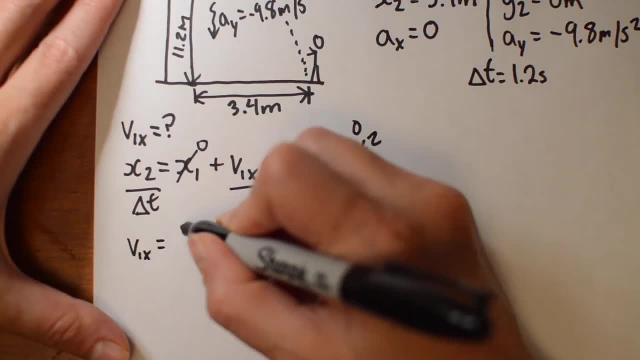 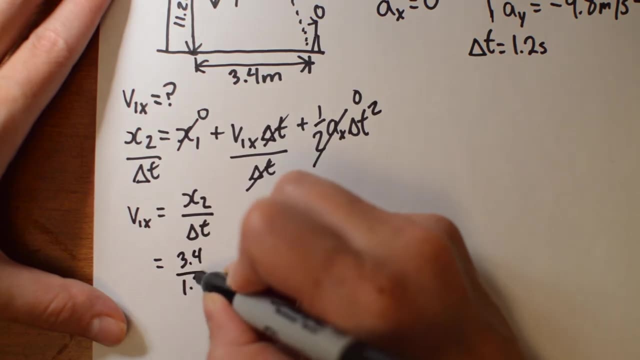 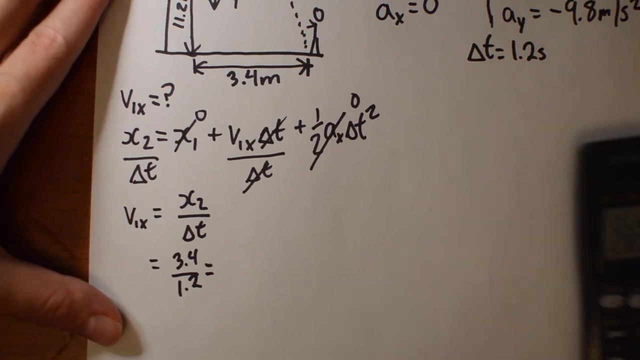 That cancels the delta t over here And I get v1x is just x2 over delta t. Plugging in my numbers, it's going to be 3.4 over 1.2, which is just 2.8.. 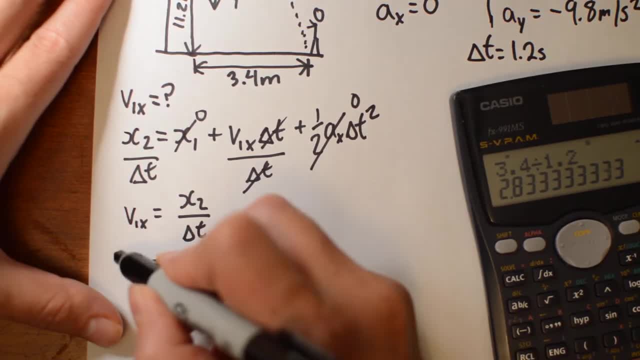 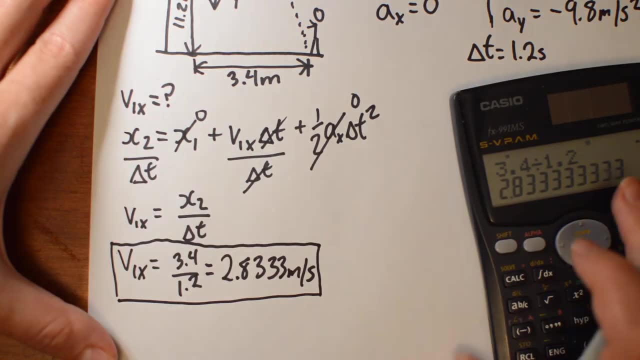 3.33 meters per second. There's my v1x. Cool, Not done there yet. I'm just going to keep that kind of on the side. Now we're going to do the same thing with y, So I want to know what v1y is. 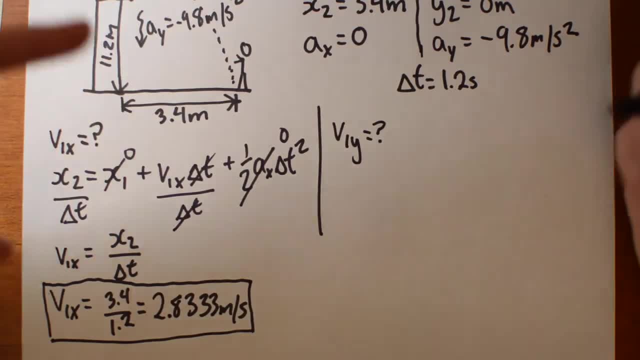 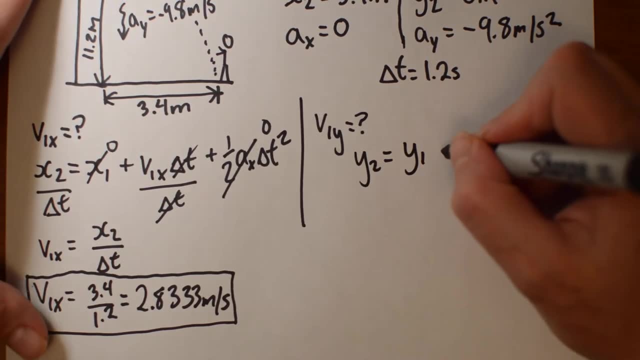 And I actually have enough information to use the same equation once again, but it's going to be a little messier because now we have an acceleration. so just a little bit more work, but it's not too bad. So y2 is y1 plus v1y delta t. 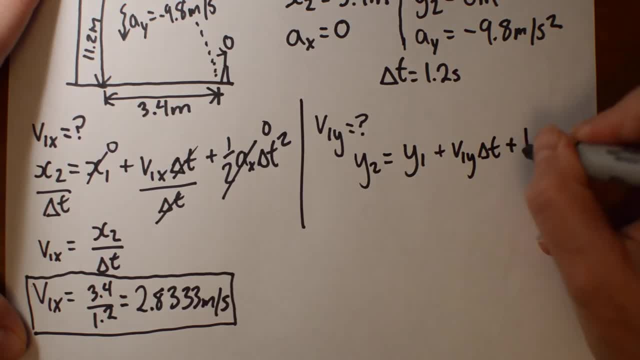 So that's the same thing: v1y delta t plus a half ay delta t squared. I'm trying to solve for v1y here. My v2y is zero, so that term is gone. I can move everything else to the other side. 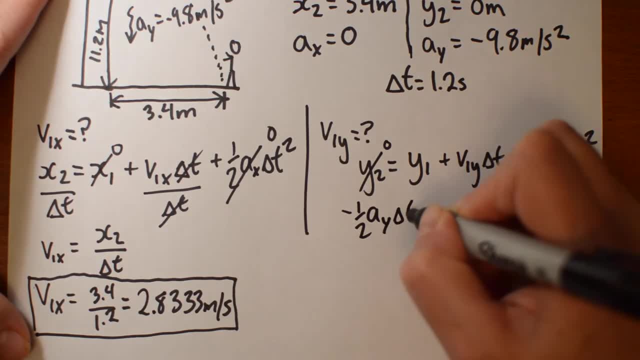 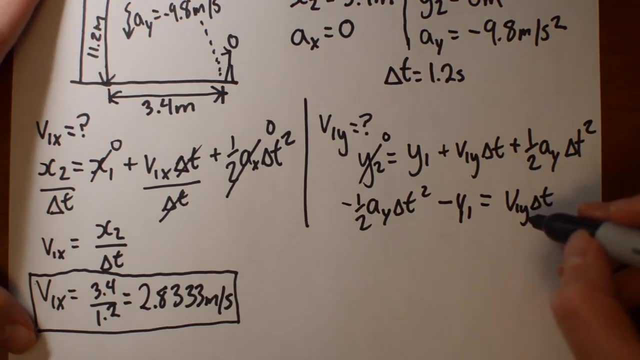 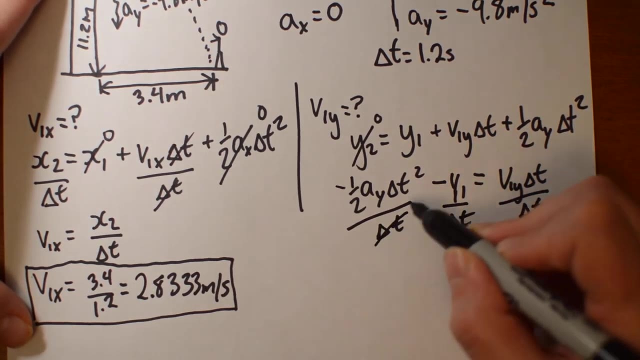 So I'll have negative a half ay delta t squared minus y1 is equal to my v1y delta t And I could divide both sides by delta t, So I might divide each term individually, Just for fun. It's nice, because then my delta t 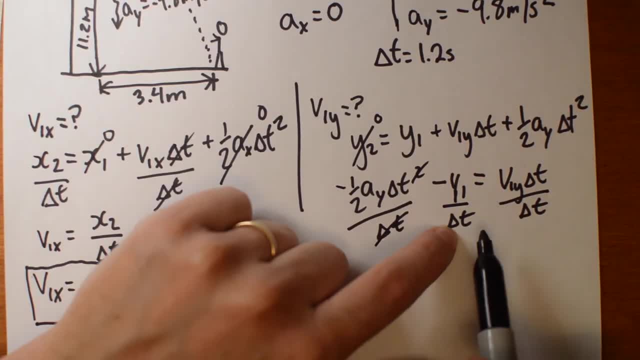 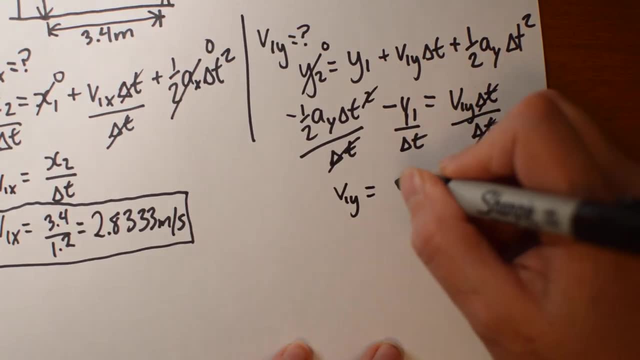 cancels one of the delta t squareds here, but it doesn't cancel this delta t here under the y1. there, Of course, these delta t's are gone, So I'll rewrite that forwards. v1y is going to be negative a half ay delta t. 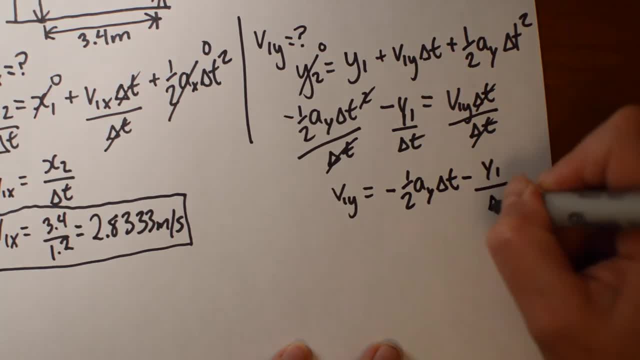 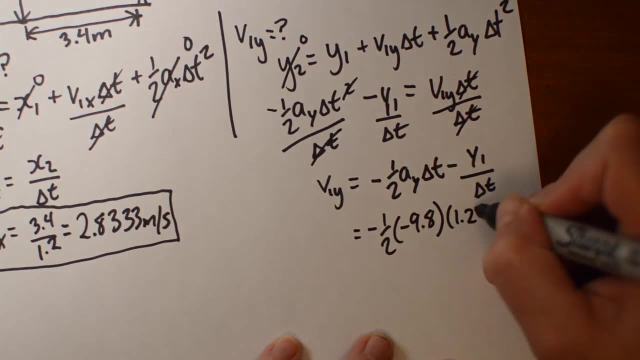 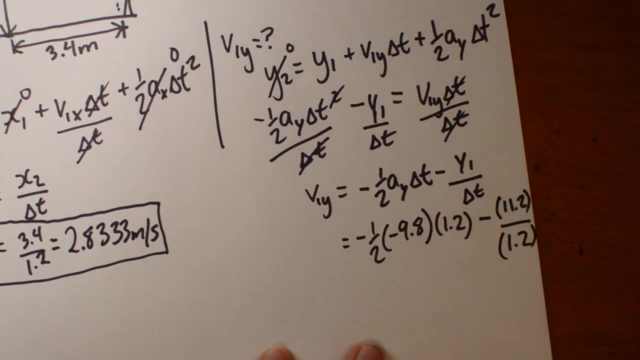 just one: delta t, not squared anymore, minus y1 over delta t, And I can plug in all my numbers: Negative, a half times negative, 9.8 times the 1.2 minus the 11.2 divided by 1.2.. 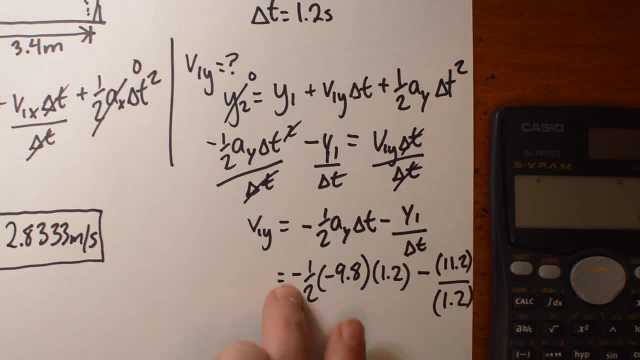 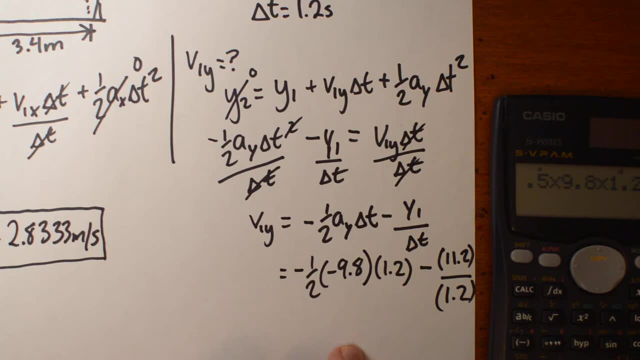 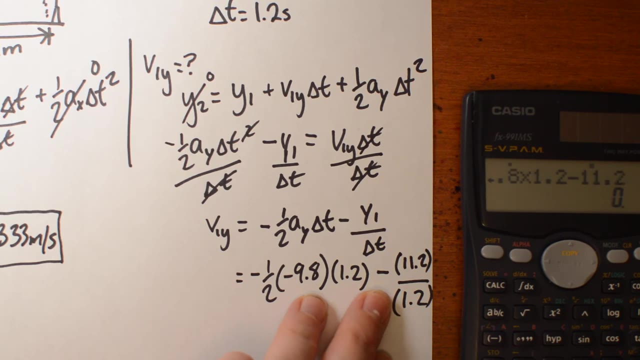 Toss that all into your calculator. So the negative a half times the negative, 9.8 is just going to make a positive. So half times 9.8 times 1.2, minus my 11.2 divided by 1.2.. 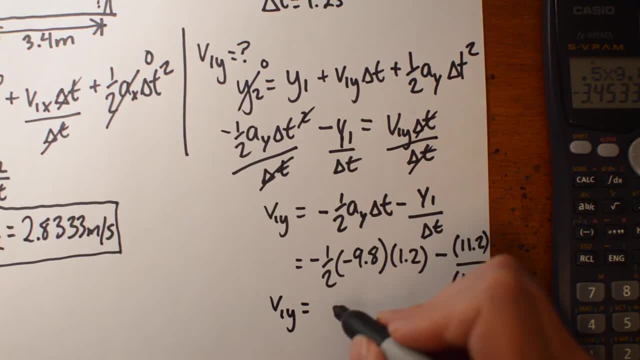 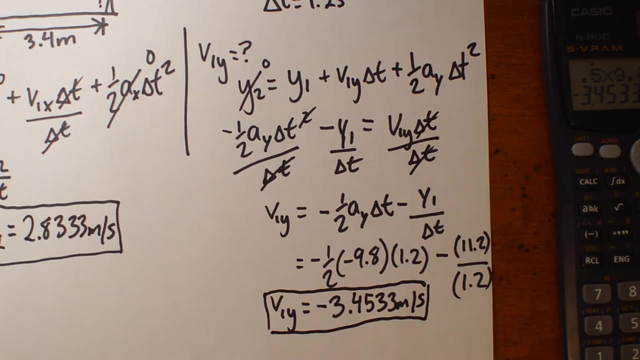 I get a v1y of negative 3.4533 meters per second. So that tells me that initially the note was kind of thrown at a downward angle. I actually didn't know that until I see that negative sign kind of popping out. 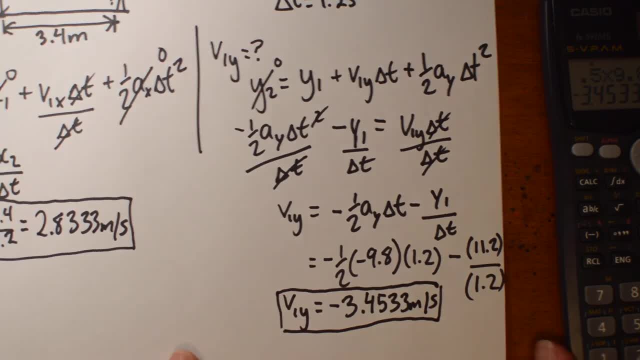 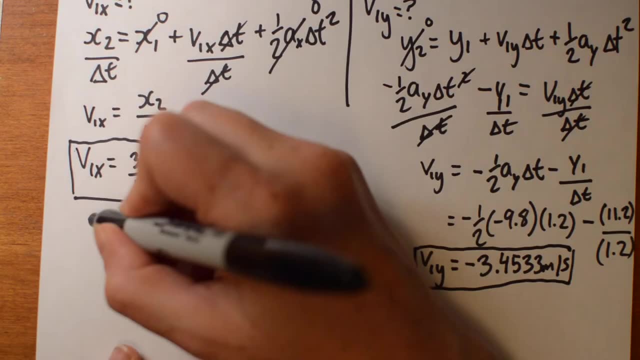 There's no way to tell from the problem. Okay, so, knowing those facts, I can put that together to get my v1, my total v1.. So there's a v1y which is actually down like this: This is v1y. 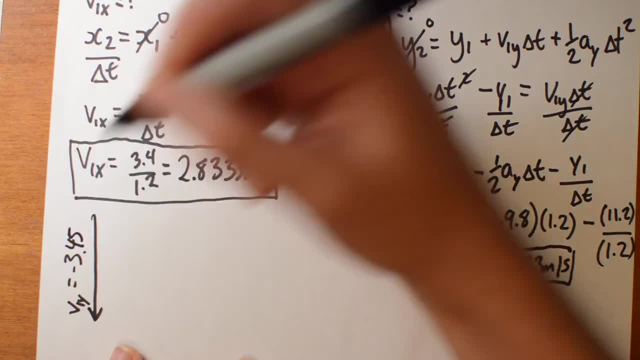 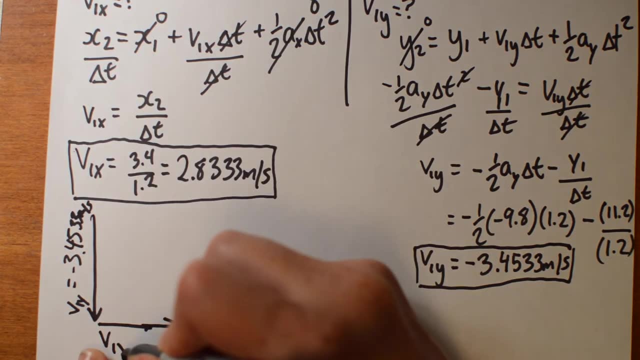 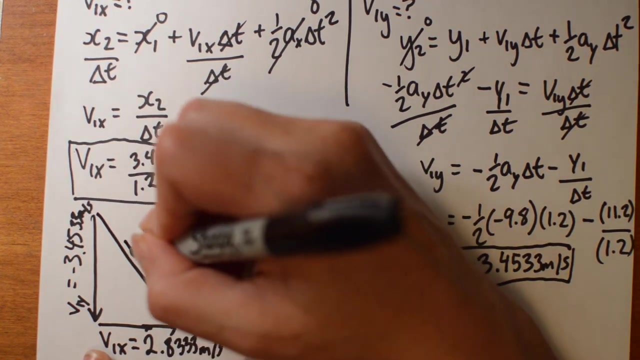 And it is negative 3.4533 meters per second, And there's a v1x which is 2.8333 meters per second, And I'm looking for the overall v1.. That's what I want to find, So I can use Pythagoras' theorem here. 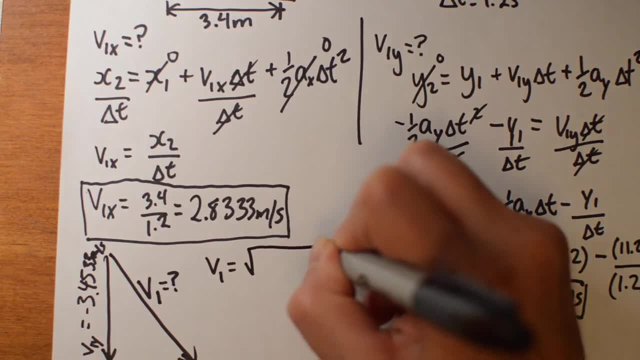 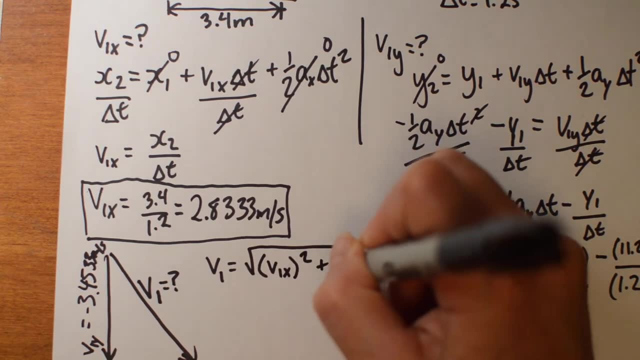 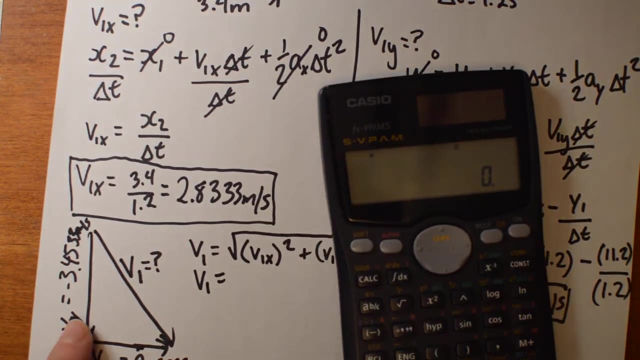 to get that v1. It's going to be the square root of the v1x and the v1y. So v1x squared plus v1y squared, Plugging all that in, I have my 3.4533 squared. 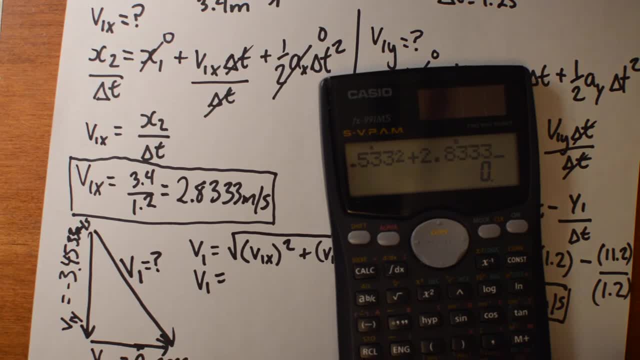 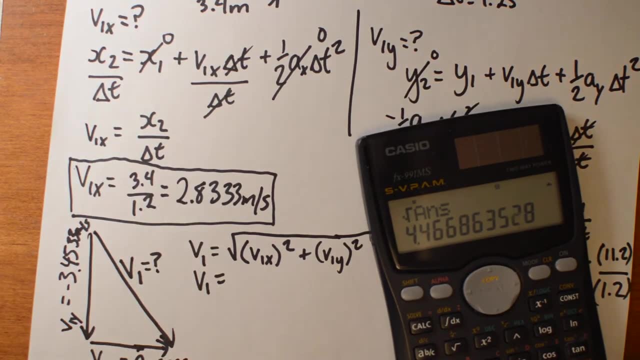 plus 2.8333 squared Square root. all that And I get a v1.. Let's check our sig figs here. It looks like 2 sig figs is my lowest number of sig figs, So I should write that as 4.5 meters per second. 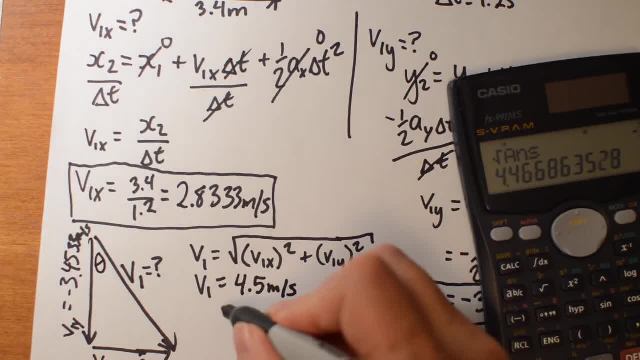 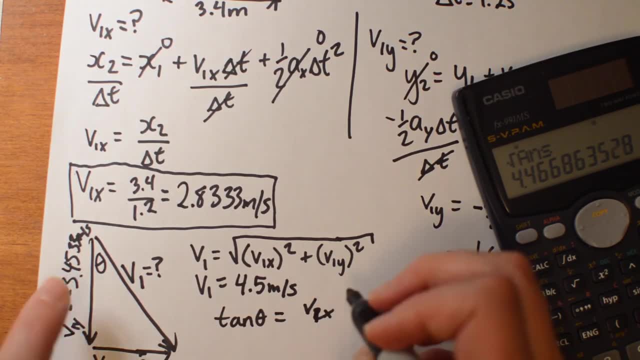 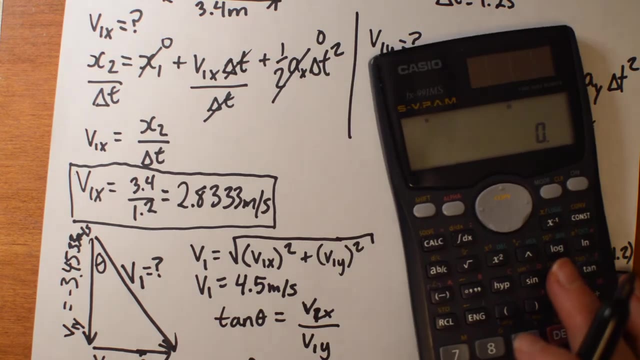 I'm not done. I need an angle. So I'll get this angle in here. Again, we can use tan, So tan of theta. This is going to be v1x over v1y Inverse tan that. So I'll do v1x- 2.8333. 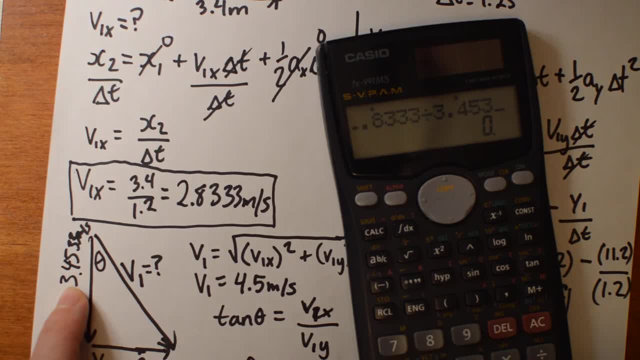 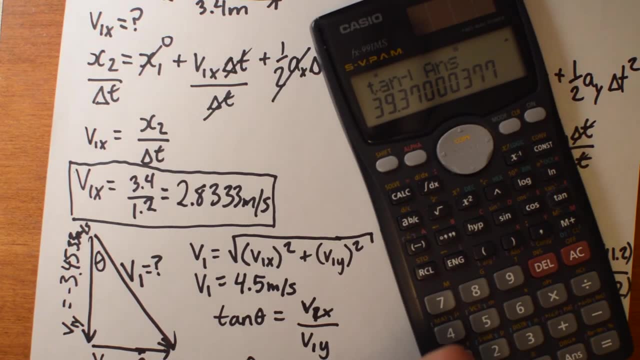 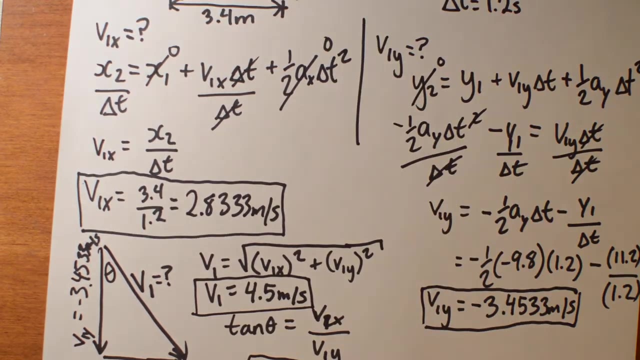 divided by v1y 3.4533.. Then inverse, tan that to get out the angle And I get 39 degrees. All right, So there's v1.. There's the angle And I've drawn the angle on my picture. And we're done.